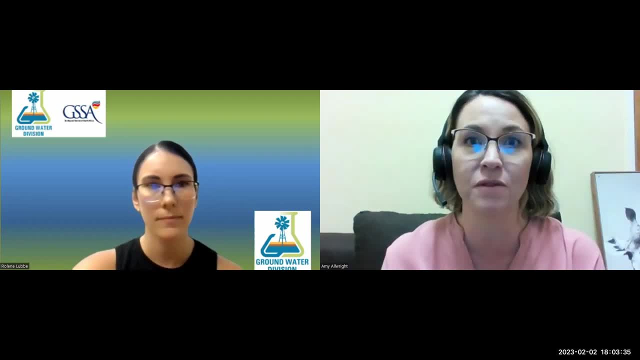 you're looking at the same problem but through a lens of, you know, from a surface water perspective. So I think it's good that we start having these talks, to like start meeting somewhere you know where these two resources meet, to start collaborating to better protect them and 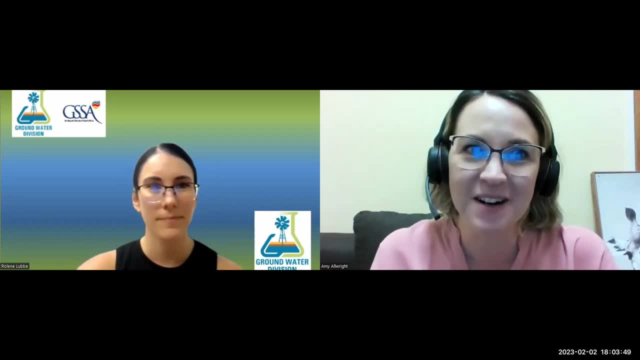 quantify and everything like that. Yeah, So welcome to everyone. I hope you enjoy the talk And with that, oh, will you please put in the chat box your name and affiliation? This talk has got CPD points, So that's just for us to take an attendance register. Just make sure that everyone gets. 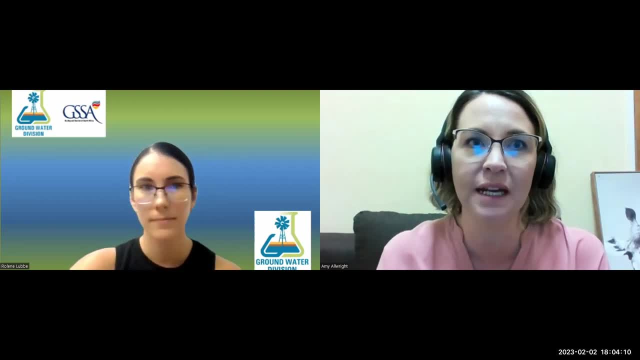 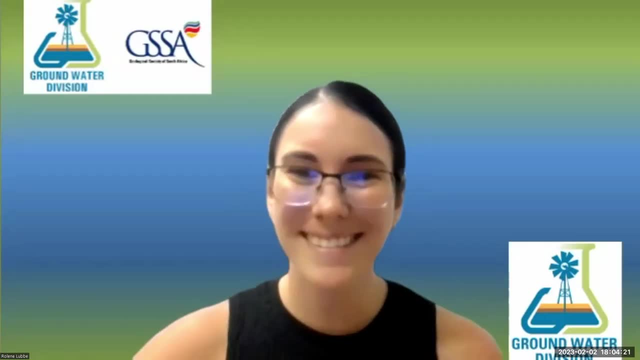 their certificate. But with that I will hand over to Eileen and she'll introduce the speaker. Thank you all very much. See you then. Hi everyone, I would like to introduce myself, Serving Daba. So I am the representative for the groundwater division. 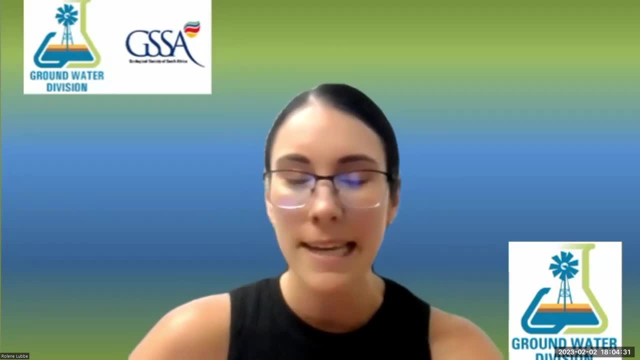 and I'm one of our professionals at the central branch, which is situated in Bluefontein. I am a full-time PhD student and research assistant at the Institute of groundwater studies at the University of Free State, And I will be introducing the speaker for today, which is Stephen Ellery. 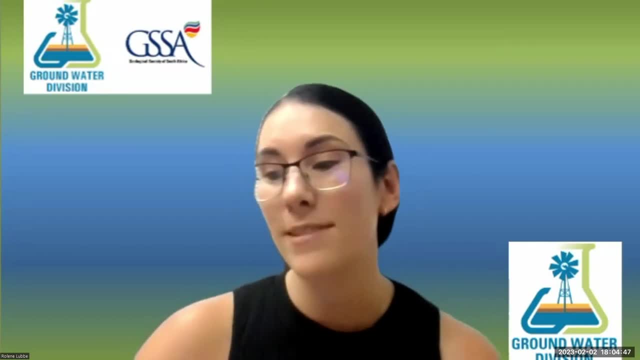 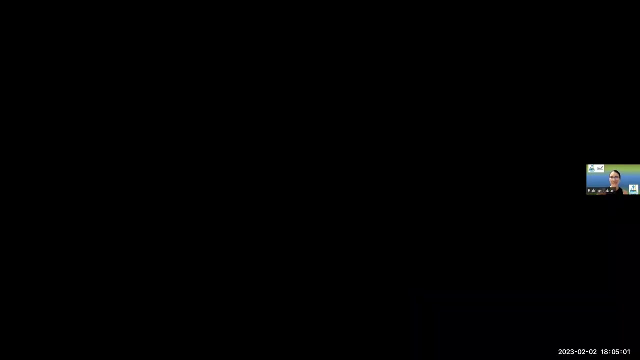 He is a Wheatland ecologist and he will be presenting World Wheatlands Day for the World Wheatlands Day presentation- Wheatlands- a friendly introduction. So I just want to provide a short introduction on on him himself. Just want to share my screen here, just the program. So Stephen Ellery is a Wheatland scientist. 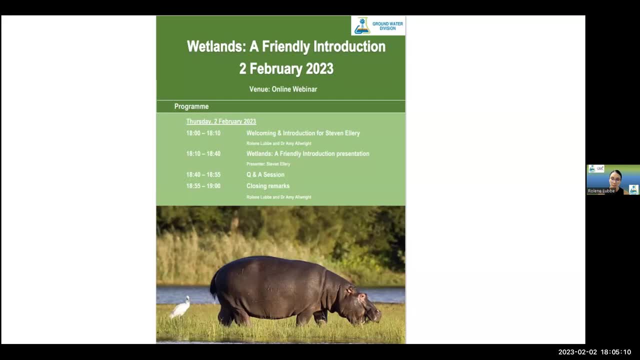 at a specialist environmental consulting firm called Ground Truth in KwaZulu-Natal. He has grown up surrounded by Wheatlanders in the Wheatlands, as his father is a well-known Wheatland researcher and educator in South Africa And he has inherited his father's passion for muddy. 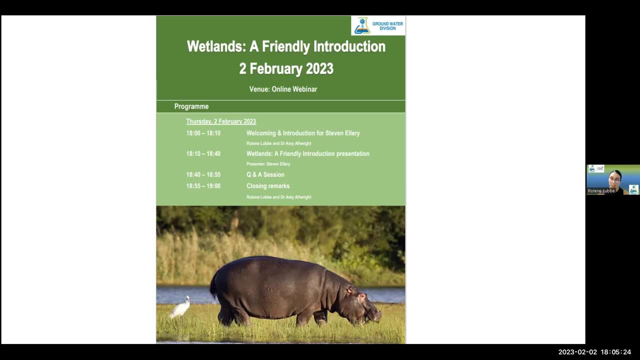 hands, swell augers and stuck gumboots. He has four years of experience, of professional experience with Ground Truth as a wetland ecologist, wetland educator and drone pilot. He has a master's degree in wetland geochemistry and geomorphology and he is a registered professional natural scientist. 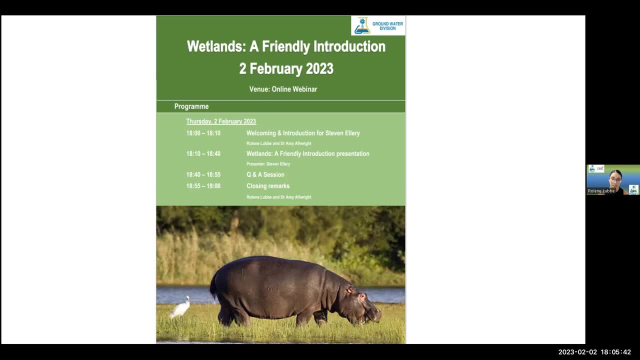 with the South African Council for Natural Scientific Professions, SACNAS. He also sits on the board of trustees at the South African Wetland Society and belongs to the Society of Wetland Scientists, which is an international wetland organization, And with that I would 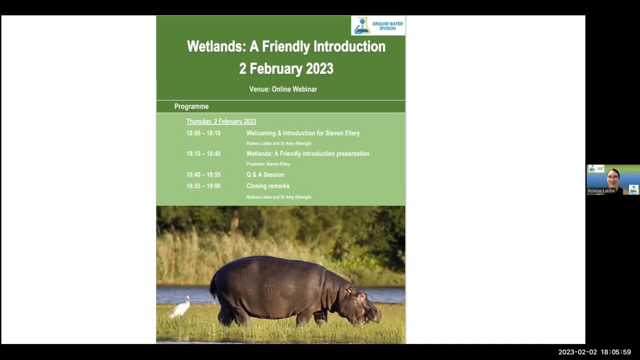 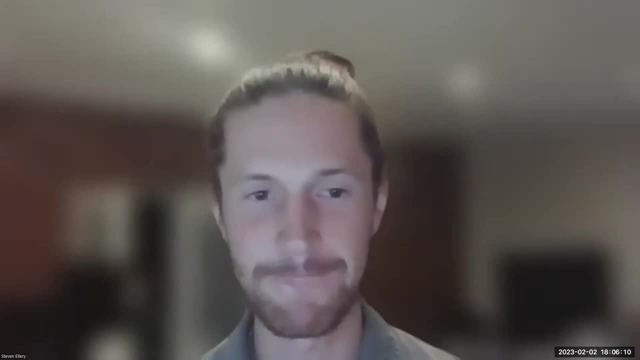 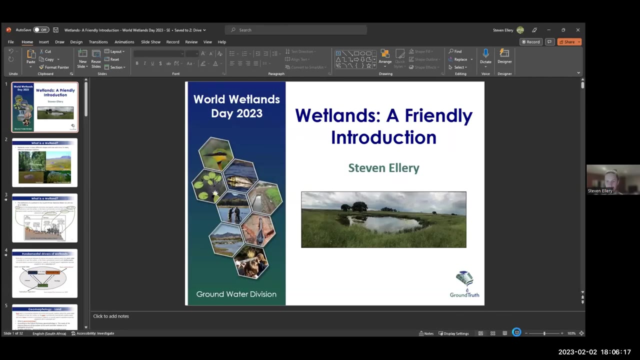 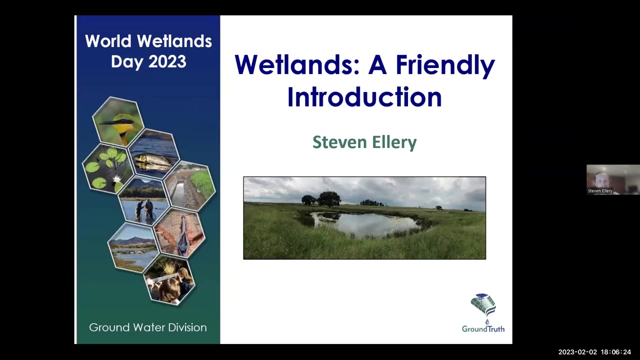 like to formally hand over to Stephen. Thank you Great. thank you so much for that introduction and it is really good to be here. Yeah, just looking at some of the names on the participants lists, I recognize some of you, which is really great. So good to be here and, yeah, I'm really. 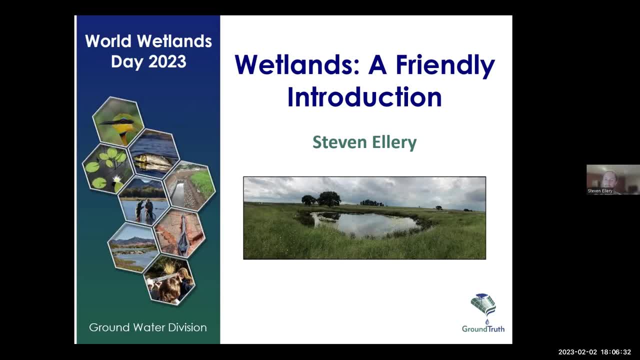 as Rowleen has alluded to, I'm really passionate about wetlands and it's something that I hope to dedicate the rest of my life to, and I really hope that with this not too scary, somewhat friendly introduction, maybe I can entice some of you guys into bringing your expertise. 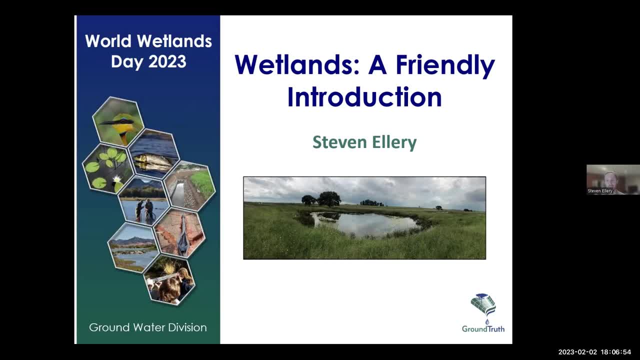 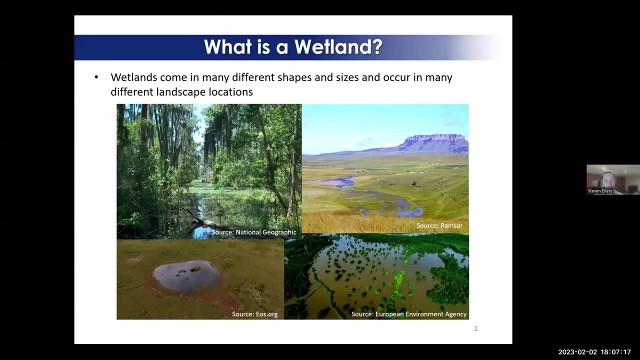 in groundwater and hydrogeology and hydrology into the wetland space, because, as you will hear, it is sorely needed. I just want to check: can everyone see my shared screen and presentation? Yes, we can see your screen, Great, cool. So without further ado, you know I'm going to go through this and maybe quickly, if there are any. 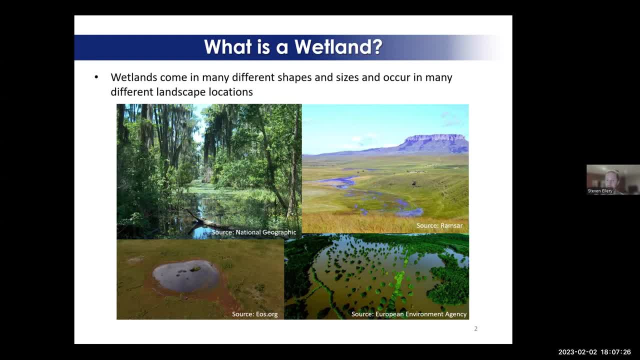 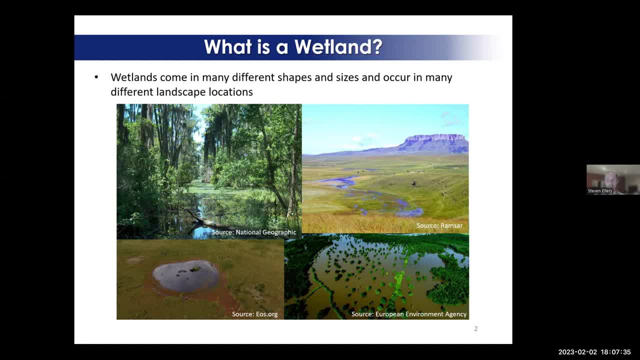 Thank you, us things. so just want to want to say that- and i might breeze through things that i assume, um, like i assume you guys know, but if i'm going too fast, please just do let me know. so, um, as you can see from these four pictures, wetlands come in many different shapes and sizes. 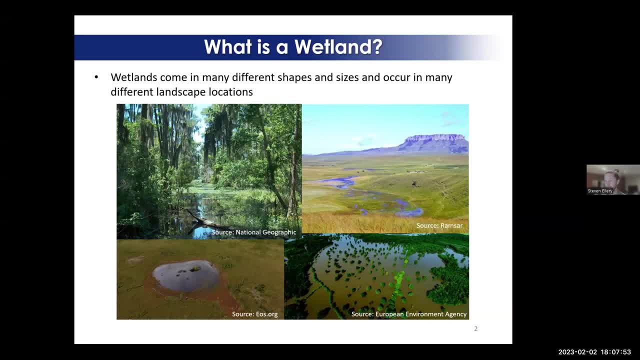 and they occur in many different landscapes and locations. so, you know, you can get a forested wetland, you can get a completely grassed wetland, you can get an enormous wetland that covers many square kilometers and you can get really really small little wetlands that are you know only. 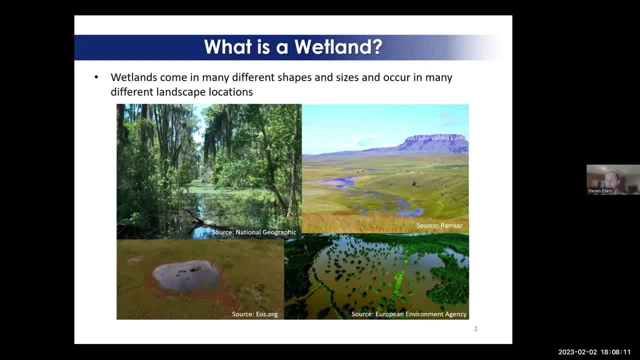 receive water from, from precipitation and rainfall. so you know they are one of the most diverse ecosystems, uh, in the world and, uh, you know they are occur all over the world. so, um, it really is quite a diverse and interesting field of practice and field study. so, in south africa, 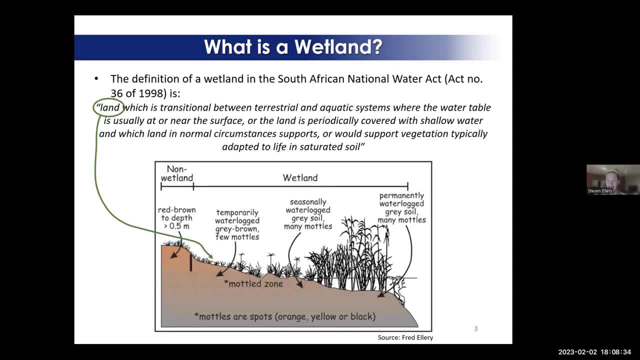 we define a wetland as land which is transitional between terrestrial and aquatic systems, where the water table is usually at or near the surface um, or the land is periodically covered in shallow water and which land in normal circumstances supports or would support vegetation and typically adapted to life in saturated soil. so i've highlighted these, these um. 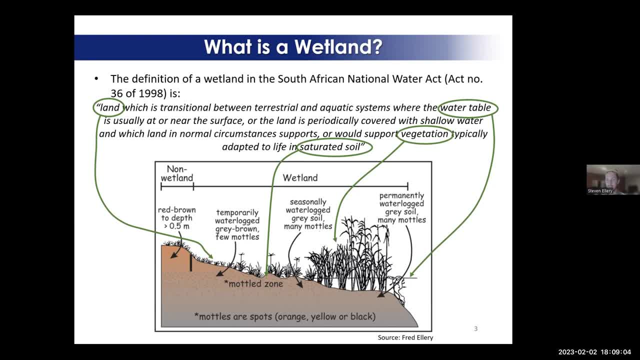 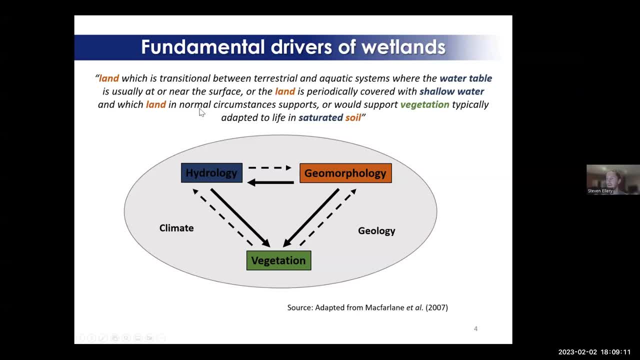 in the bottom right-hand corner of this definition and we're going to just take a little bit of a deeper dive into what these actually look like and what they mean and how they interact. so you can see- i've colored and the definition according to um, this little conceptual model that 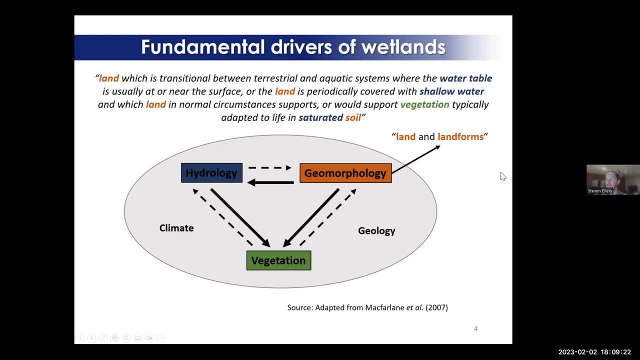 i have here. so first we're going to look at geomorphology, and that really speaks to land and land forms, and we're going to take a deep dive into into each of these aspects of the fundamental drivers of wetland origin and wetland formation. so geomorphology refers to land and land forms. 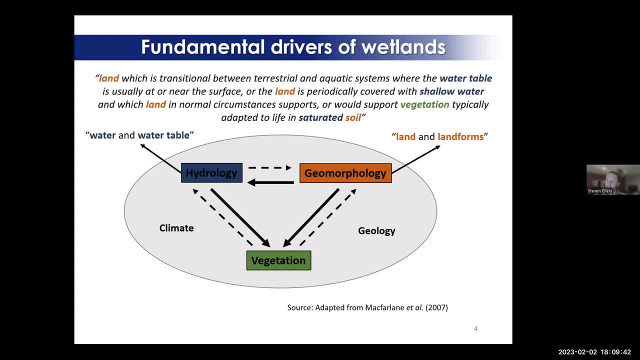 hydrology, i'm sure most of you know, refers to water, either surface or groundwater, as well as the water table, and vegetation refers to, in a wetland context, hydrophytic vegetation or vegetation that is adapted to living in saturated soils and then around these three components. 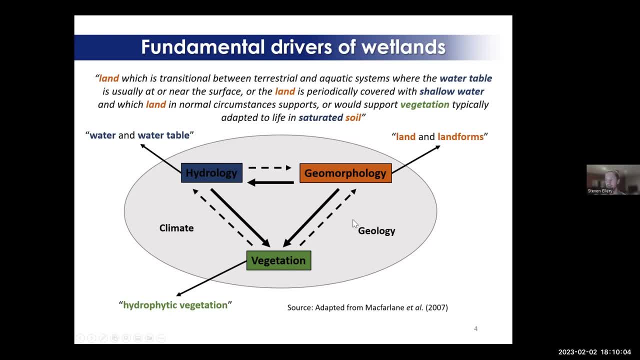 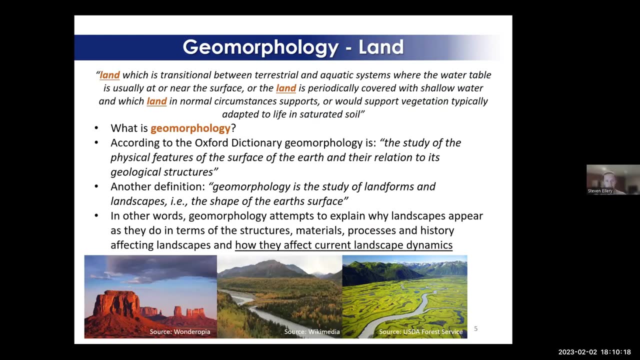 you will see that there is climate and there is geology, and both of which play to a lesser degree but an important role in the formation of wetlands. so what is geomorphology? according to the oxford dictionary, it's the study of physical features on the surface of the earth and their relation. 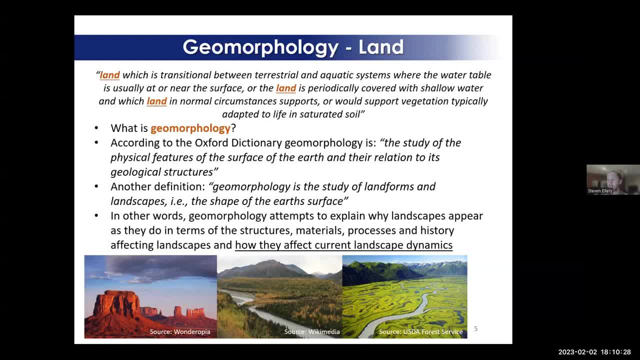 to its geological structures, or another definition that maybe i prefer is it's the study of landforms and the shape of the earth's surface. so really, in other words, it attempts to explain why landscapes appear the way they do, um, and how they affect current landscape dynamics, and i'm sure you know. 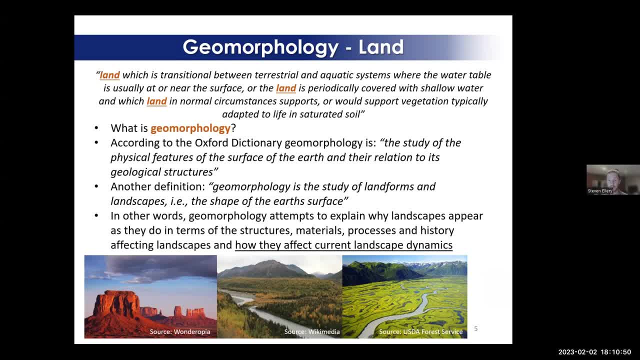 if we imagine a valley, for example, um it it is the. you know, the bottom of the valley is the low point in which water typically correct collects, and and that valley bottom is the surface of the earth's surface. so i'm just going to jump back and forth a little bit. 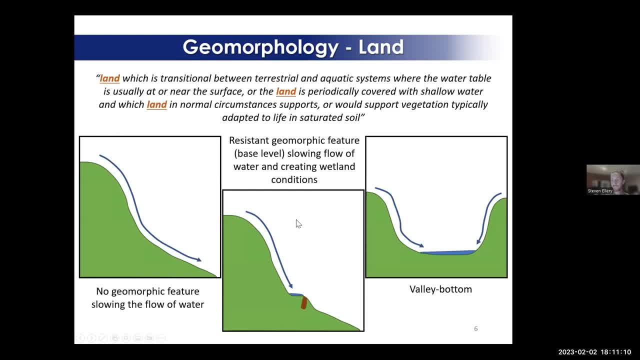 um, and so the idea is that geomorphology is a geomorphological structure. now, geomorphological means structure, so i'm just going to let you go through this. um, so geomorphology, um, i'm just going to take a little bit of time to go through this. so this hill slope and is a geomorphological 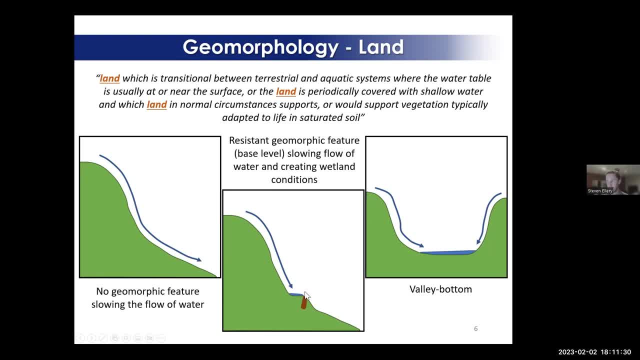 structure and when water falls on top of the hill, it will naturally, because of gravity, a resistant geomorphic feature, which we, as wetland scientists, call a base level, which is resistant to erosion and therefore may slow the water down And it may act as a 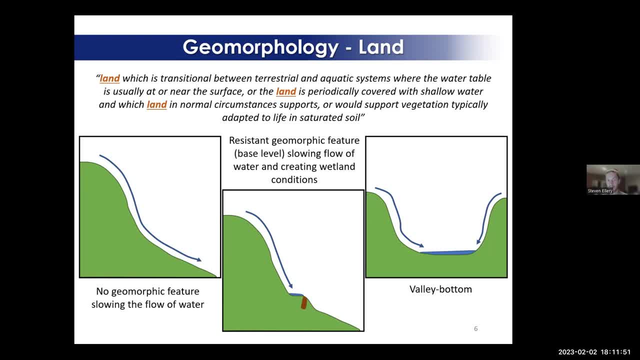 base level, or a nick point, as we also call it, to create conditions that are conducive to wetland formation, And this is something that happens all the time And we'll talk about this a little bit later. But also on the right hand side here you can see a valley bottom And, as a geomorphic 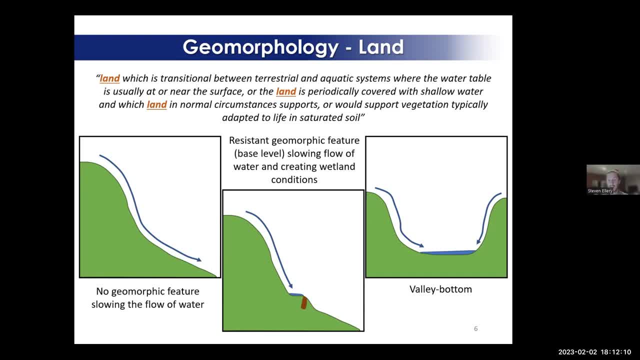 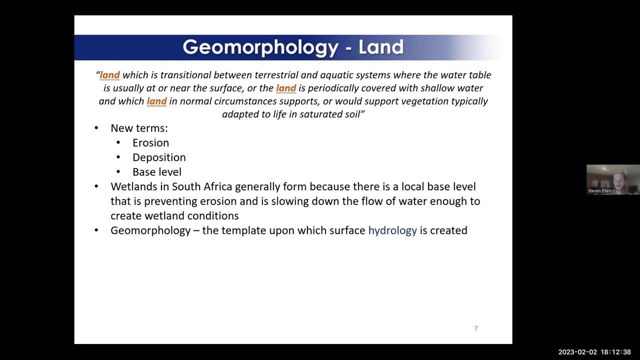 feature. that is typically where water collects, And those geomorphic features often result or are formed as a consequence of geology, lithology, as well as hydrological movement over those land surfaces. So yeah, some new terms. maybe not new to all of you, but erosion is the movement of soil or sediment. 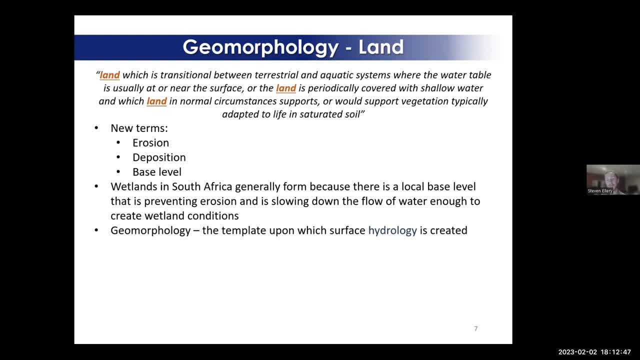 or land from one place to a place where it is deposited and where deposition takes place, And through that process of erosion and deposition wetlands often are found, And we'll talk about this in an example a little bit later. But in South Africa typically wetlands form because there is a local base level. 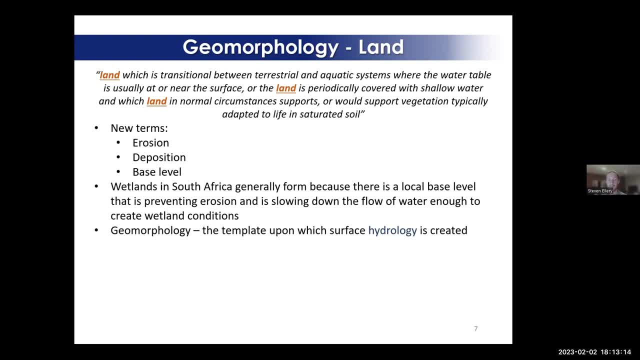 that is preventing erosion and is slowing down the flow of water enough to create wetland conditions. So in a sense, geomorphology as a whole and the geomorphological landscape in South Africa is more than a single geomorphological landscape, But geomorphology can be thought of as the template. 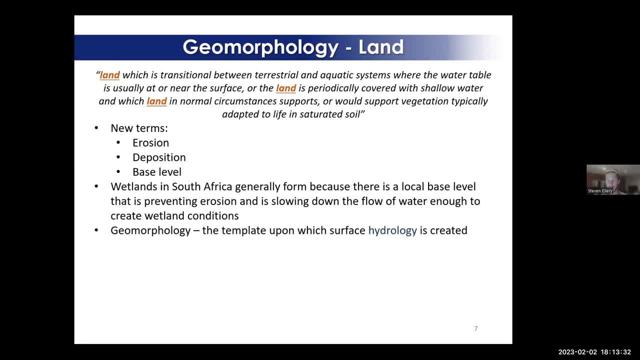 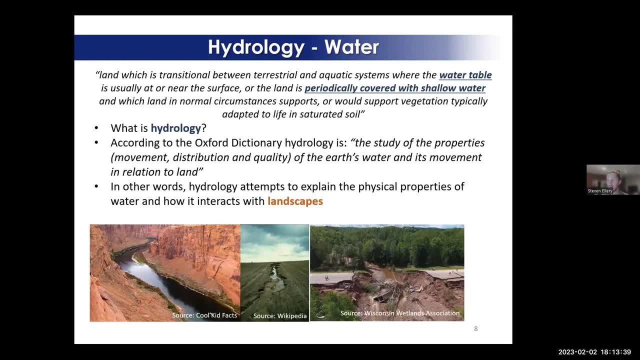 upon which surface hydrology wetlands is created. So what is hydrology? Well, according to the Oxford Dictionary, hydrology is the study of properties which are the movement, distribution and quality of the earth's water in relation to its land. So you can see. 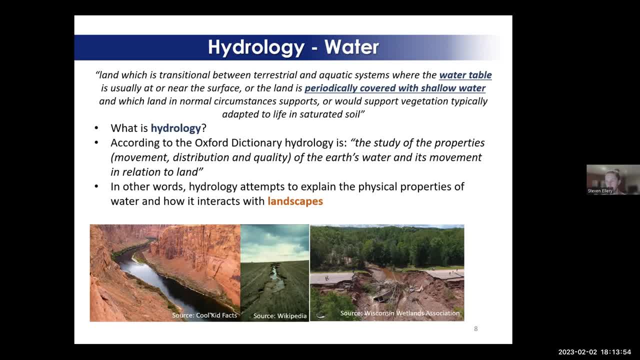 already that there's a link between hydrology and land surfaces. So hydrology is a way of. So hydrology attempts to explain the physical properties of water and how it interacts with landscapes. And you know, I'm sure we're all aware- of some of the flooding that's happened in KwaZulu-Natal last year and this year- well, last year mostly. 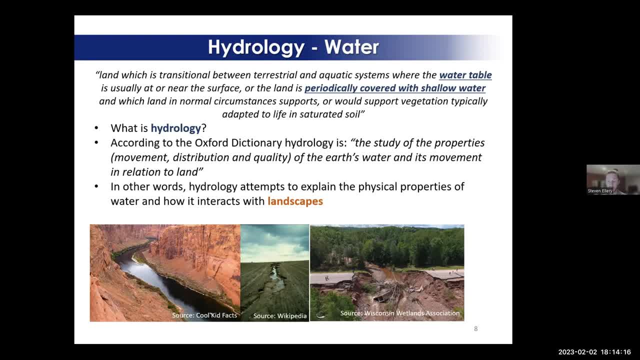 And we also, you know, I'm sure that just speaks to the power that hydrological processes can have if they aren't managed properly or well. And you know those hydrological events, those floods, are often a consequence, or, you know, partially a consequence, of changes in the landscape and the geomorphology of the surrounding landscape and the catchments of those systems. 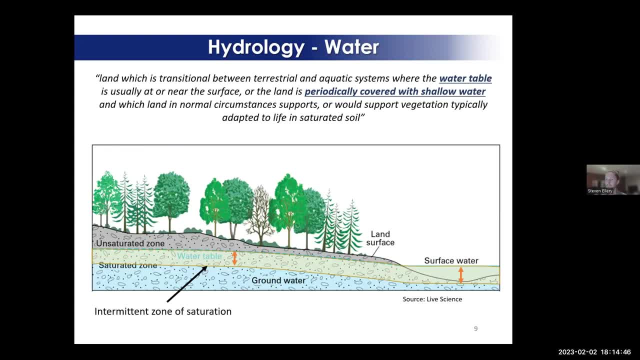 So here we'll talk a little bit about how groundwater and surface water interact to form wetlands. So wetlands, as we see in the definition, are aquatic systems where the water table is usually at or near the surface, And we'll talk about this. but we define wetlands as when there's water within the top 50% of the surface. 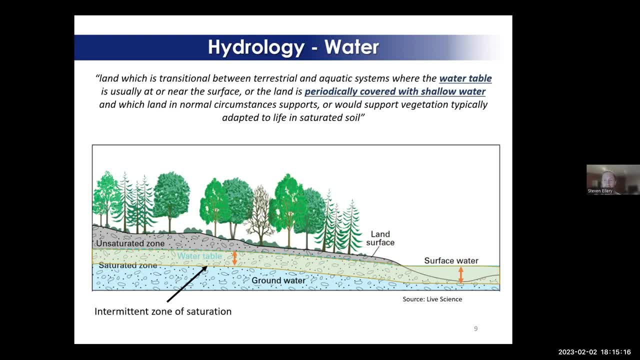 So that's 50 centimeters of the soil surface. Anything below 50 centimeters- typically wetland plant roots- can't reach that and therefore you actually get a movement away of hydrophytic vegetation when the water table is below 50 centimeters below the surface. 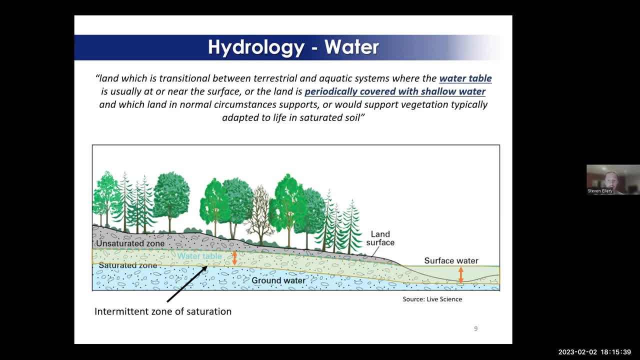 So, as I'm sure you will know, the water table fluctuates depending on various factors such as rainfall conditions, lithological features and fractured geologies, etc. So wetlands form in areas where the water table is above or near the ground level and, generally speaking, the interaction between wetlands and groundwater is poorly understood in the South African context especially. 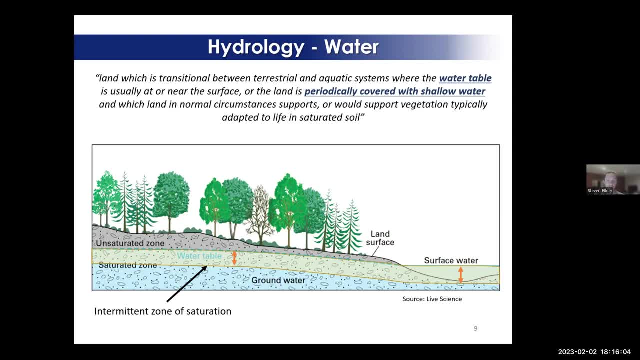 as it has not been a focus of many research questions in the past. However, there has been a recent focus and a recent uprise in the understanding of this interaction, and there have been many more studies that are being done to unpack the interaction between wetlands and surface water. 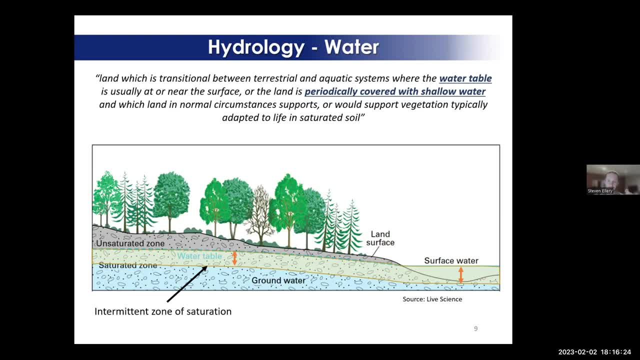 So you know this is a subtle call, or not so subtle call- to you guys as hydrologists and groundwater specialists to consider, you know, asking more questions about: well, how do groundwater features contribute to wetlands and how do wetlands contribute to groundwater features? 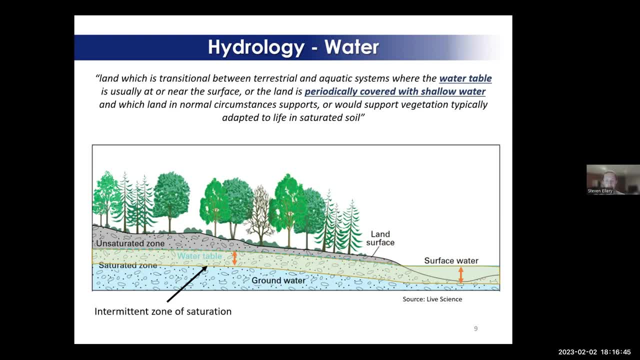 You know, but it is generally understood that many wetlands are supported by local groundwater recharge, through interflow and through the presence of local perched aquifers. And I'm sure a lot of you know that certain geologies have strong groundwater linkages. you know, in geologies where there are 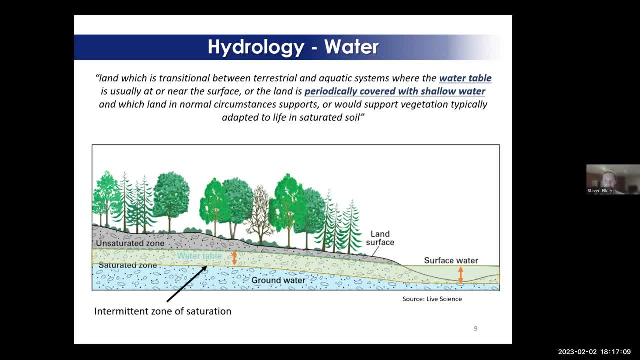 a high occurrence of fractured or fractures within geology, And it is often assumed that wetlands found in those areas are at least supplemented by groundwater. But again, this is not always certain and there's a lot of research to do in that space. 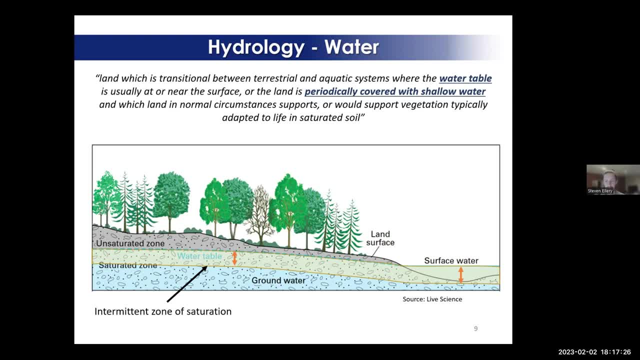 But a well-known example of a wetland complex- and we were chatting about this wetland complex just before the course started- is the Isimangaliso wetland complex, or the, you know, towards Lake St Lucia, And that wetland complex falls on the coastal plain where there is a very strong ground-surface water interaction. 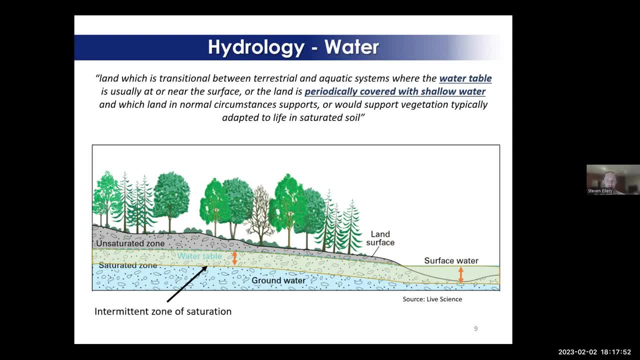 You know. further to that, many wetlands are known to recharge local and regional aquifers and can often contribute to the hydrological inputs of groundwater systems. A great example of this would be the Cromwell wetland in the Eastern Cape, which is known for its prolific contribution to the local and regional aquifers there. 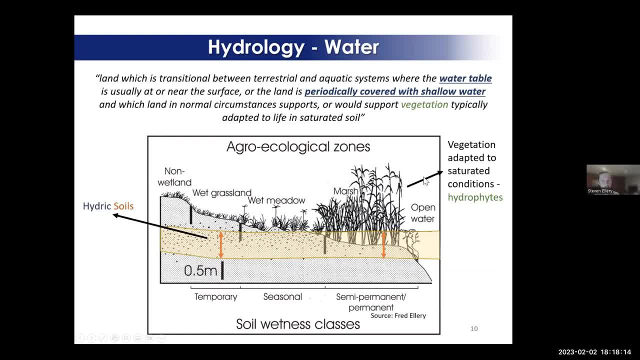 So to move on, you know, as I mentioned before, typically we define wetlands as areas where the top 50 centimeters of the ground is saturated for enough time for the soils to produce what are known as hydromorphic soil features or hydric soils. 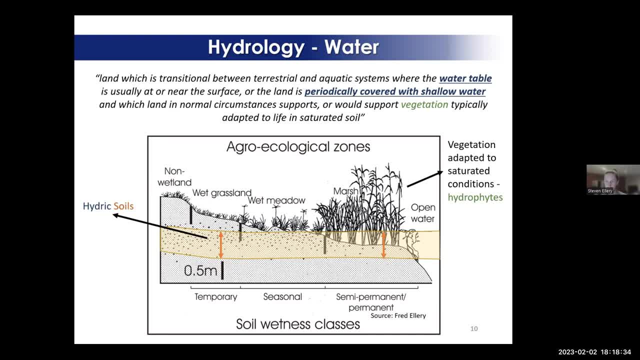 And these features include, but are not limited to, glade soils, so basically where all the color drains out of the soil and that also results in the formation of what are known as mottles, basically small ion or manganese reductions within the soils, And that is a result generally of fluctuating water tables. 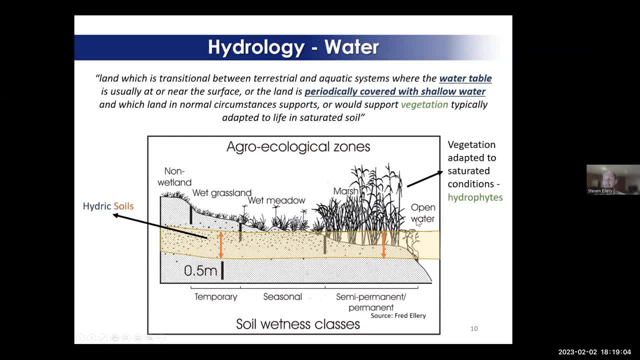 As the water table rises towards the surface, iron and magnesium and manganese go into solution, and as that water table drops and as oxygen is reintroduced to the soil profile, those elements are precipitated out of solution and they create these small nodules called mottles. 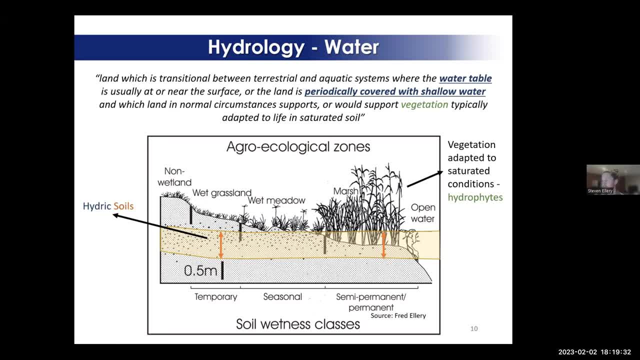 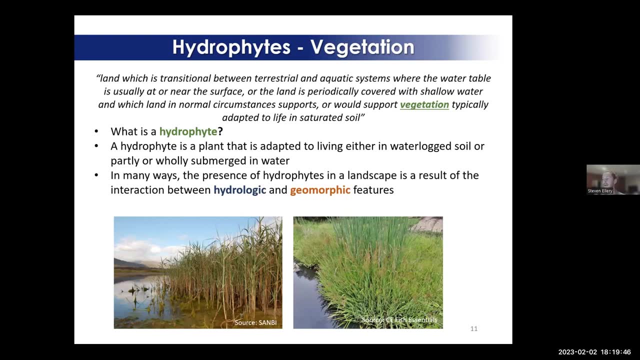 And then another feature to identify wetlands is, of course, vegetation that is adapted to saturated conditions, aka hydrophiles. So a hydrophile is a plant that is adapted to living in either waterlogged soils or completely submerged soils. So in many ways, the presence of hydrophiles in the landscape is a result of the interaction 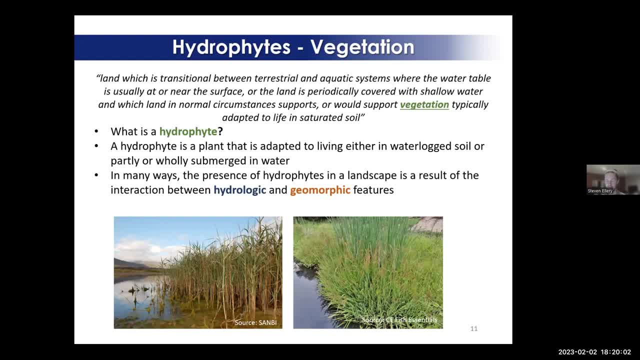 between hydrologic and geomorphic features, And hydrophiles are often used as effective monitoring tools to detect and assess changes in hydrologic and geomorphic features in the landscape, And they can show change in a matter of months, So you know if, all of a sudden, a dam is built on a wetland or upstream of a wetland, for example. 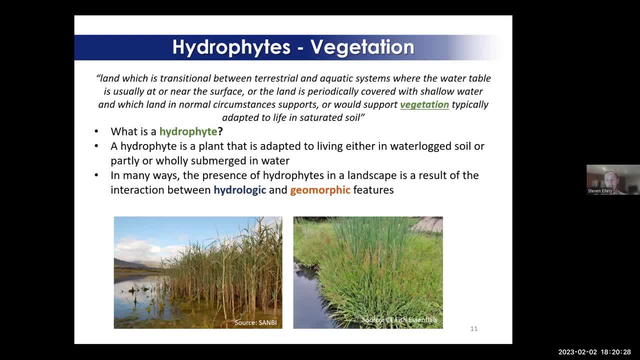 the yeah, the drying up or the holding back of that water will be reflected fairly rapidly in the vegetation signatures in that wetland. So many wetland vegetation indices or indicators have been created as a surrogate measure of wetland water quality, as well as wetness regimes within a wetland. 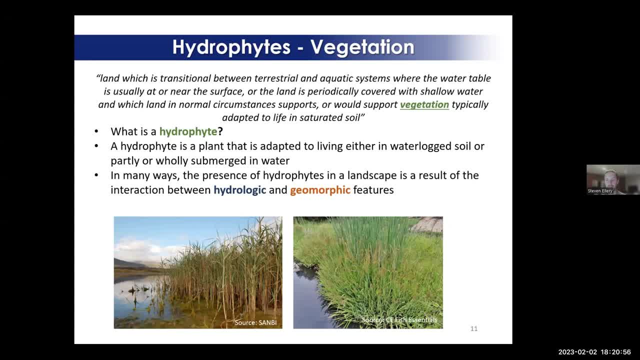 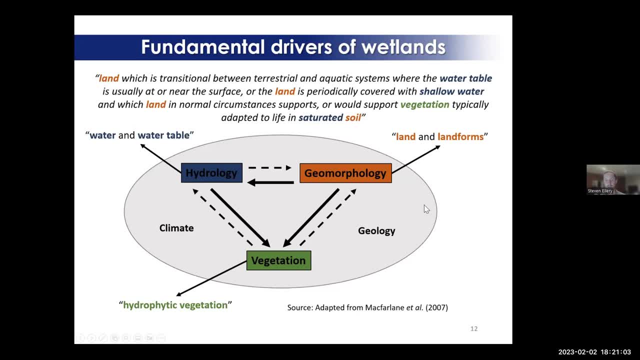 And just to say I'm not monitoring the chat at all, So if there are questions coming in the chat, please let me know. Yeah, So to come back to this conceptual diagram, we can see that there are dark arrows and dashed arrows. 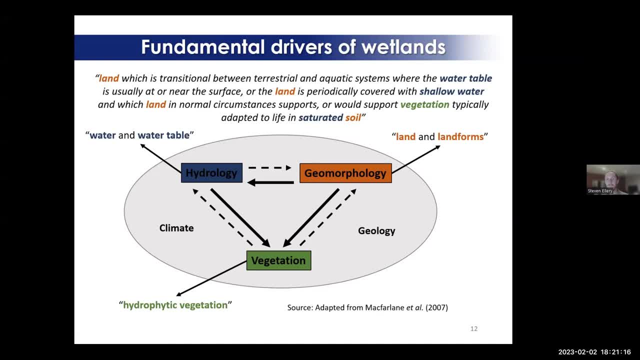 So a dark arrow in this conceptual diagram represents a very strong influence. So we can see that geomorphology has a very strong influence on how water moves. It moves across and through the landscape And hydrology has a weaker influence on geomorphology. 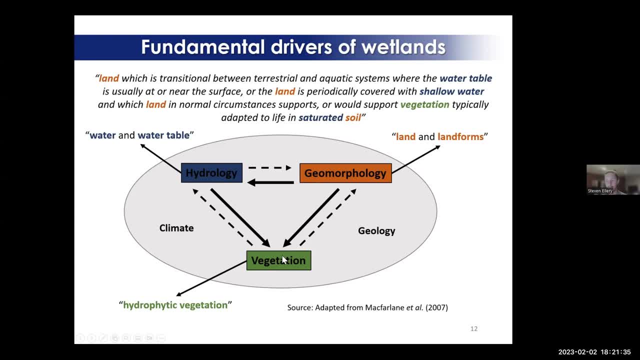 And hydrology and geomorphology. both have a very strong influence on vegetation and the type and the composition of vegetation found within a wetland And vegetation has a weaker feedback on hydrology and geomorphology. And just to note something that took me a while to get used to: 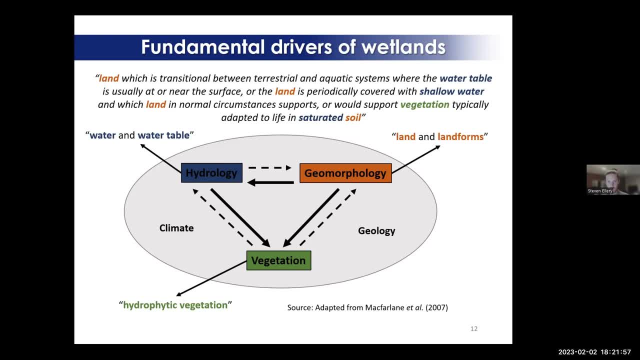 But really helped in my understanding of these three drivers Is that typically, when we consider geomorphology as a science or as a discipline, we talk about a time scale or a temporal scale that is just much greater than hydrology or vegetation. So you know, we talk about millions and millions of years of the evolution of the landscape. 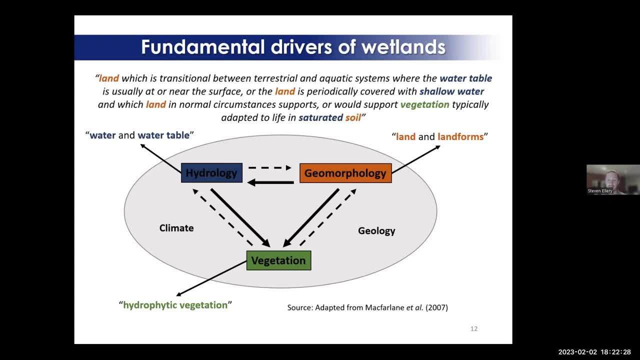 Being shaped by different processes, you know, sometimes tectonic processes and large uprise events in the case of South Africa, And when we talk about a hydrological scale, that time scale that we generally consider is much shorter. So that's why I always like to use geomorphology as kind of this benchmark. 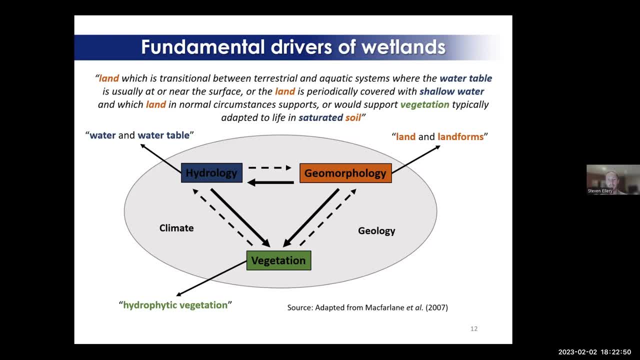 As kind of this base template upon which we can then start building our understanding of a wetland, And then adding the hydrology on top of that, and then adding the vegetation on top of that, And then after that you know human impacts like water quality issues and things. 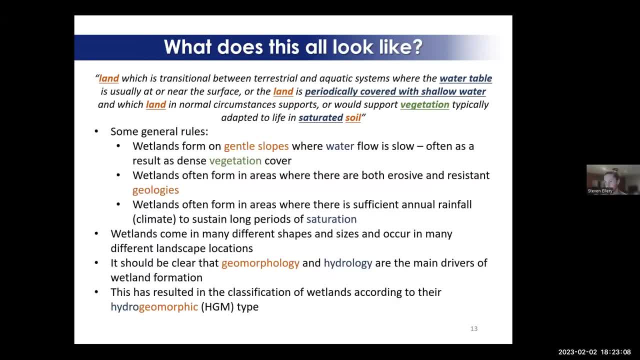 Which we will talk about just now as well. So what does this all look like? actually, Some general rules. Wetlands form on gentle slopes, Often where water flow is slow and often as a result of dense vegetation. Wetlands often form in areas where there are both erosive and resistant geologies. 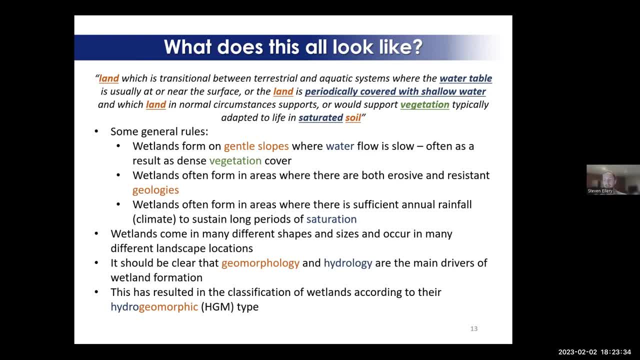 So the resistant geology forming a base level and allowing for the erosion upstream of that resistant geology To form flat and gently sloping conditions, With wetland formation, And wetlands often form in areas where there is sufficient annual rainfall, Which is as part of that conceptual model of the climate aspect. 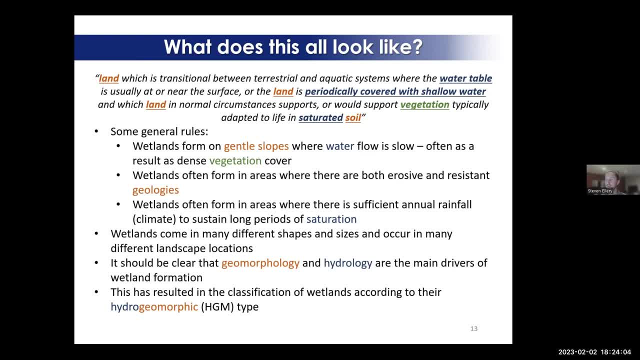 To sustain long periods of saturation. Wetlands also come in many different shapes and sizes, And it should start becoming clear to you that geomorphology and hydrology are the main drivers of wetland formation, And this has resulted in a classification system of wetlands according to what we call the hydrogeomorphic type. 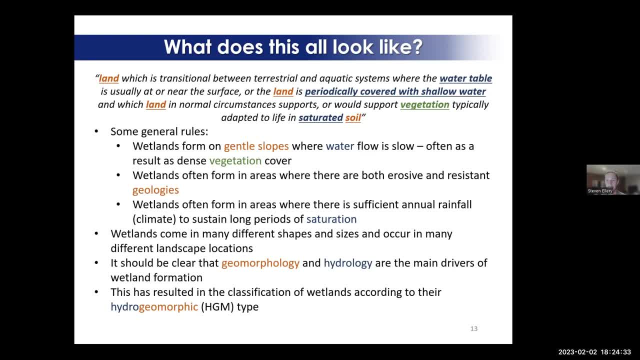 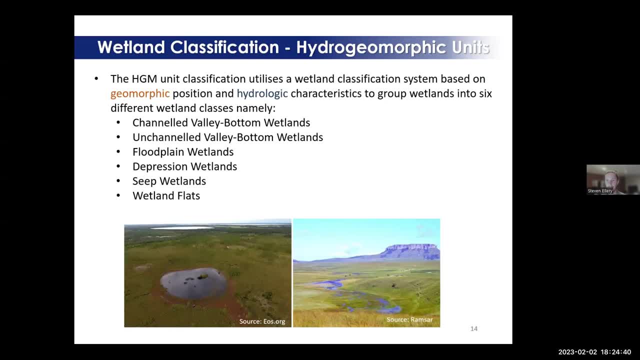 And so the hydrogeomorphic type, or HGM unit classification as we call it, Utilizes a system that is based on the geomorphic position of that wetland, As well as the hydrologic characteristics of those group of wetlands. So the widely used HGM- 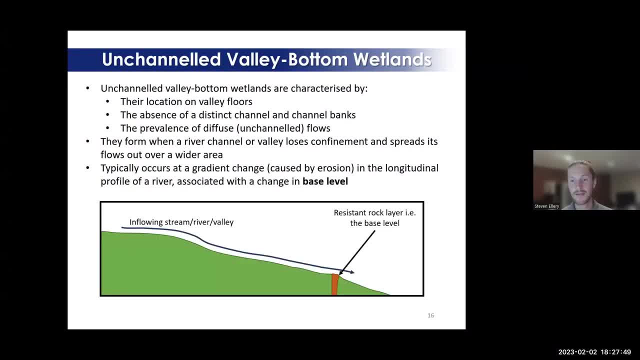 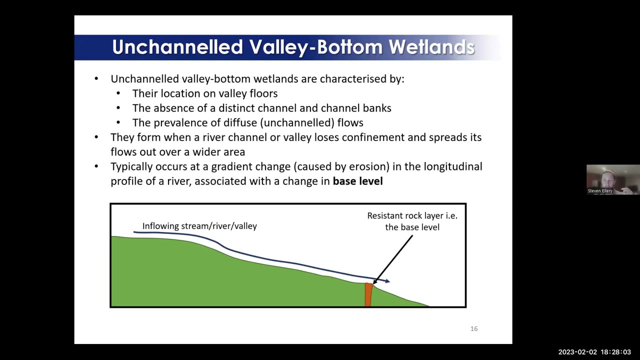 If we take this example again of a resistant rock layer or base level At the toe of a slope And with water flowing over that hill slope, If the discharge of that water is too great for the slope, It will result in erosive conditions. 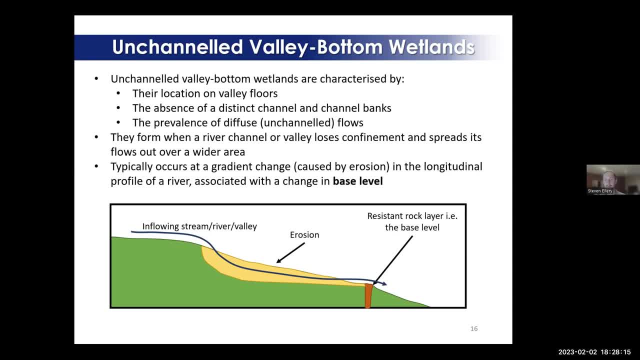 And basically the cutting out of that hill slope Until the discharge from the catchment is appropriate for the slope of the wetland. And once this process has occurred You will see that there's a much more gentle slope upstream of that resistant rock layer or base layer. 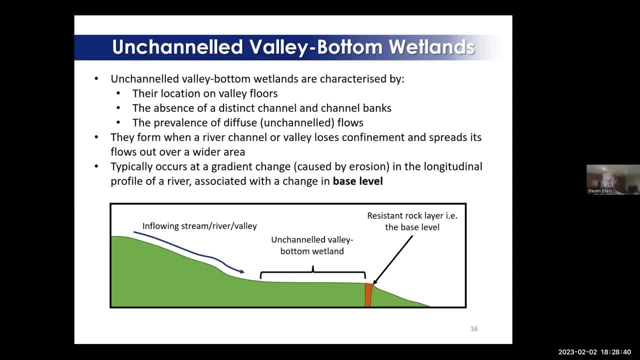 And that's a very typical way that an unchanneled valley bottom wetland forms in the landscape. And again, when we're thinking of this geomorphic process, This can happen over hundreds of thousands of years. And if we think about how quickly we can put a drain into an unchanneled valley bottom, 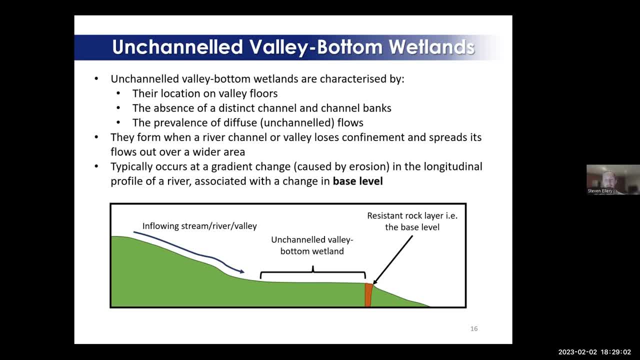 In a matter of days We completely undo those hundreds of thousands of years of work that has happened And create that unchanneled valley bottom. So also just a call to us to really consider our impact on the environment. Of course I feel like I'm speaking to the converted here. 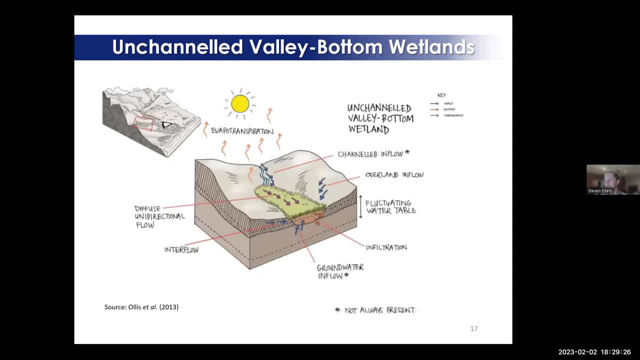 But yeah, So the conceptual model generally, Or just more, the inflows, outflows and flows. You can see that typically, You know there is a channeled inflow into an unchanneled valley bottom. Once it hits that unchanneled valley bottom, 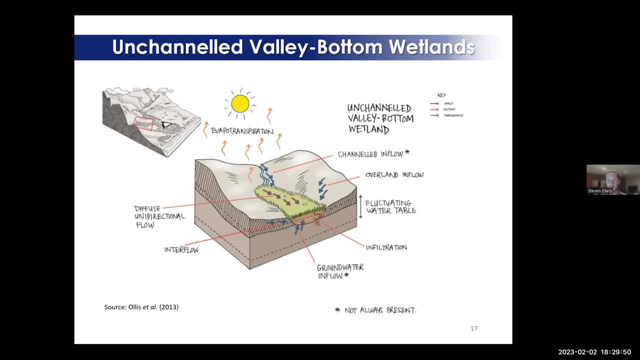 The through flow is typically characterized by diffuse flow, Often in the direction of the slope of the wetland. Generally unchanneled valley bottom wetlands receive interflow from lateral inputs, So from the valley side As well as overland flow from, you know, surface hydrology coming into the wetland. 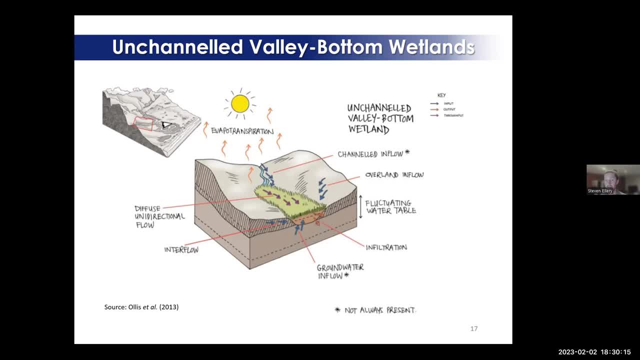 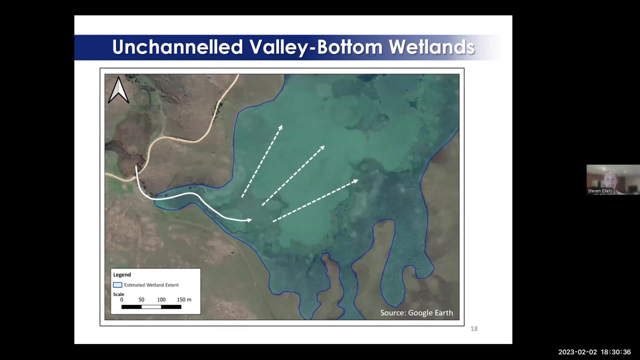 And also typically they are characterized by infiltration, So they can often act As groundwater recharge points, Sometimes as groundwater inflow. So one of my favorite wetlands in the whole world is the Amgeni Flay Here in KwaZulu-Natal. 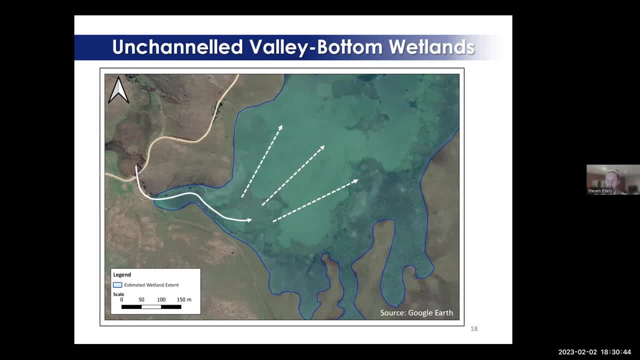 And it is one of the most spectacular examples of an unchanneled valley bottom And you can see here that there's a channeled flow coming in And as it hits this massive, Very, very flat And valley bottom, It just spreads out into this really incredible, incredible wetland. 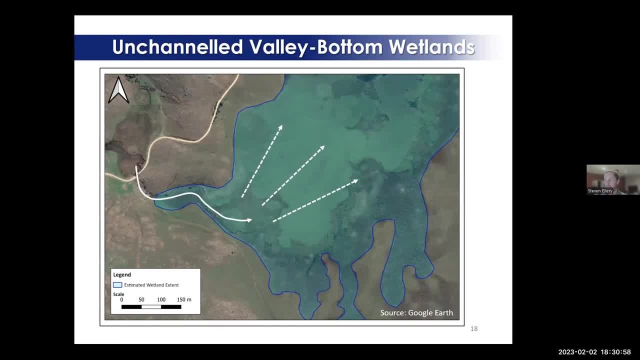 So, yeah, If you ever have a chance to go to the Amgeni Flay Nature Reserve, I really encourage you to go and have a look. It's yeah spectacular, And there are just many wattled cranes And blue cranes. 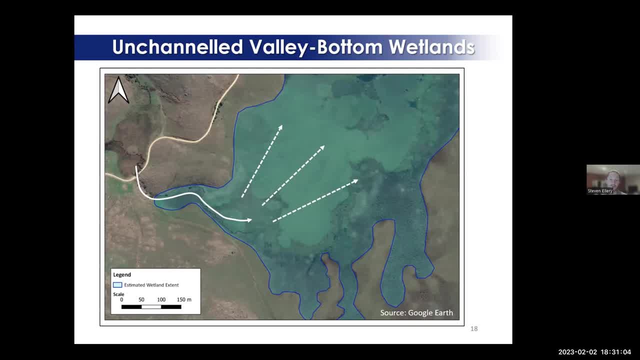 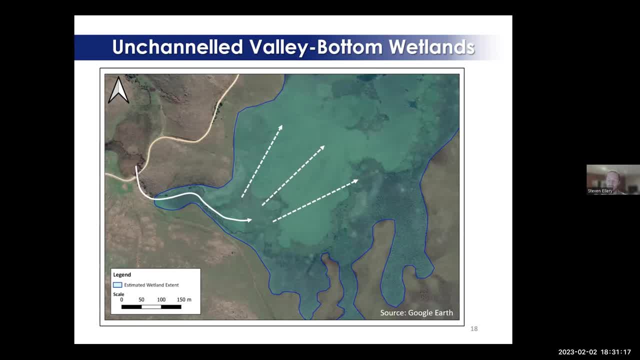 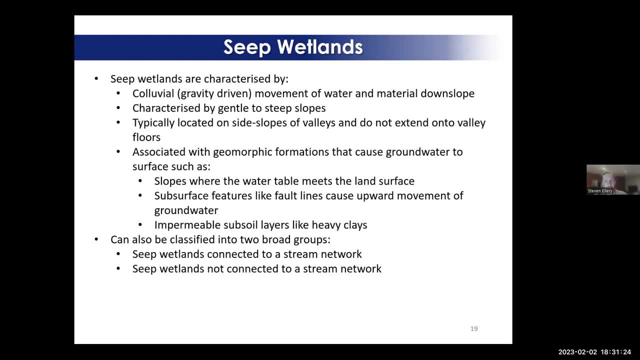 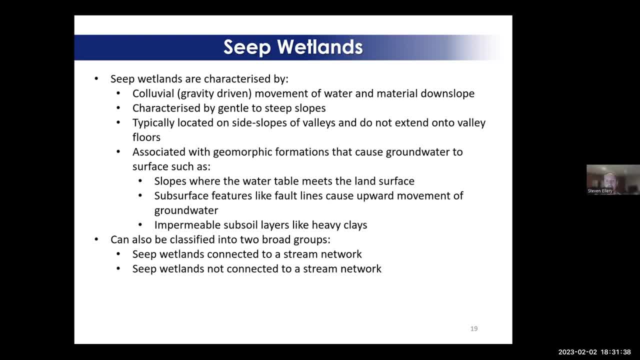 of Wetland timeline. So typically throughout lands are found on striking steeper and gradients and they are often driven by the movement of water downslope And and and that can be characterized by a gentle true sleep two, two very steep slopes. 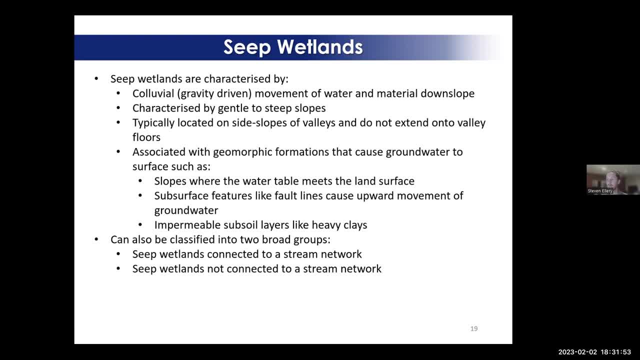 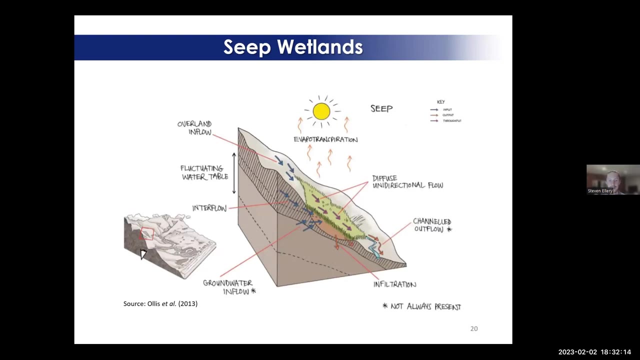 with geomorphic formations. quite often that cause groundwater to surface, So often they're associated with a resistant lithology or a perched aquifer that forces groundwater out onto the surface, creating a seepage wetland. So just a quick example of a conceptual model of a seeped wetland. 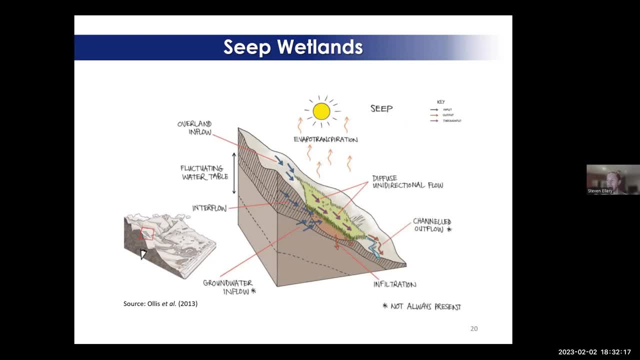 They are often contributed to by overland flow, but typically most of the the flow that enters or surfaces in the seep wetland is through interflow, and then often there's groundwater contributions as well, And here's an example of a seepage wetland with a small spring at the head and again. 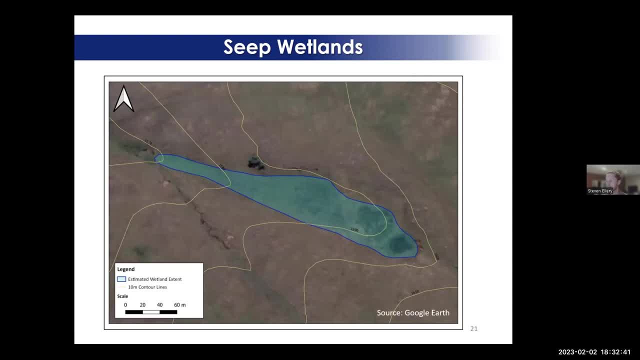 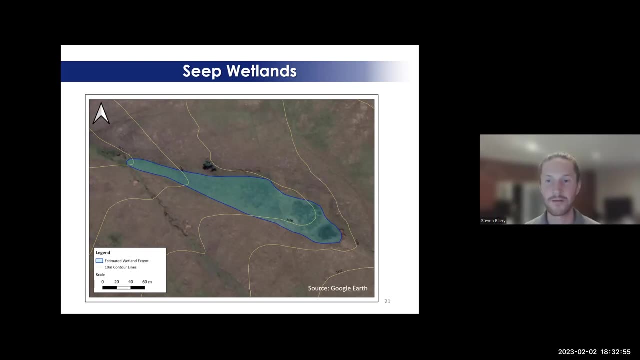 you can see just by these contour lines that the gradient is fairly steep, So you can see that there's a lot of water in the water. But, yeah, there are hydrological conditions, ie groundwater contributions, which are allowing for this wetland to persist in the landscape. 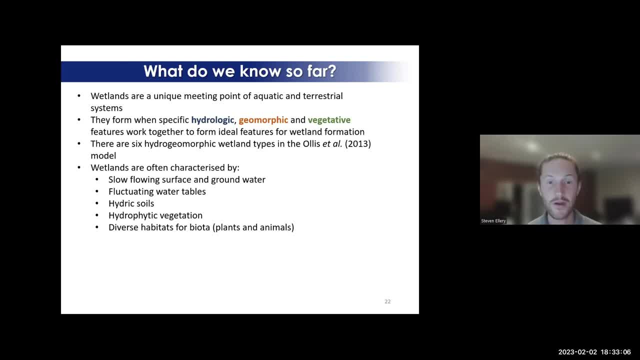 So what do we know so far? Wetlands are a unique meeting point of aquatic and terrestrial systems and they form when specific conditions work together or features in the wetlands. So what do we know so far? Wetlands are a unique meeting point of aquatic and terrestrial systems and they form when specific conditions work together or features in the wetlands. 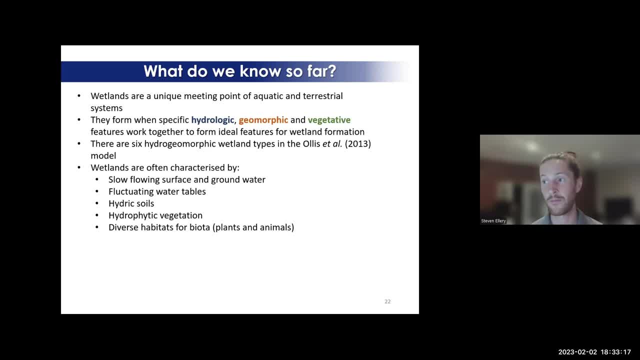 work together to form ideal conditions for wetland formation, And we spoke about two of the HGM unit types as defined by Dean Arliss, and they are often characterized by slow flowing surface and groundwater, fluctuating water tables, hydric soils, hydrophytic vegetation and diverse habitats for biota plants and animals. 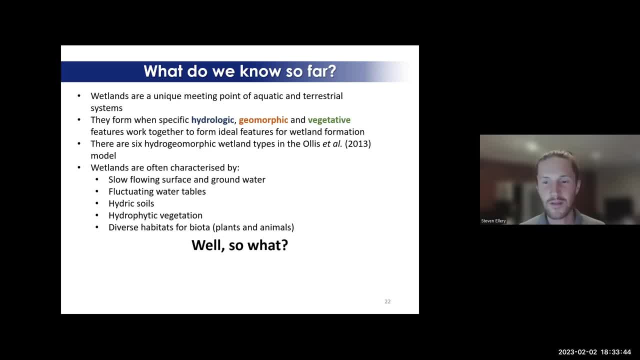 Now some of you might be thinking: well, you know, so what? Why should I care about that? and it's just water and land and plants. Well, wetlands provide us with trillions of dollars of ecosystem services completely free of charge. We don't have to pay for any of it. 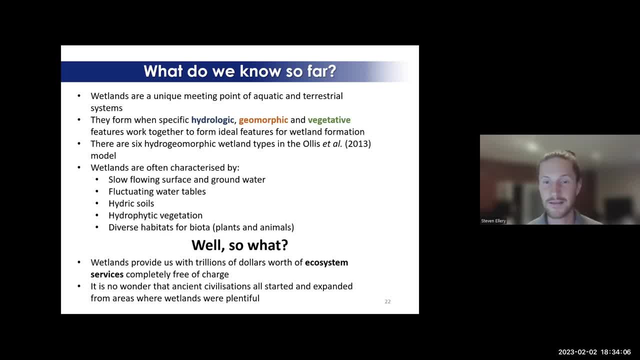 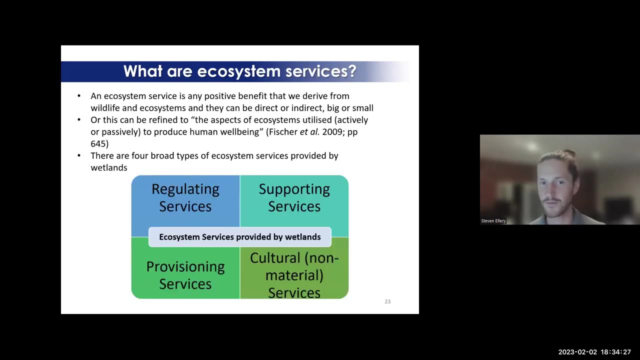 And so it's no wonder that ancient civilizations such as the Egyptians, such as some of the great and Middle Eastern civilizations, expanded or started and formed themselves, and expanded from areas where wetlands were plentiful. And so I mentioned ecosystem services. What are ecosystem services? The definition that I really 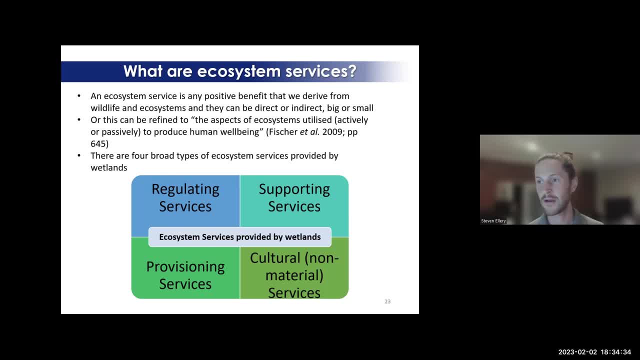 like is the aspects of ecosystems that are utilized, actively or passively, to produce human well-being, And when we consider ecosystem services, we typically think of four broad types of ecosystem services, namely regulating, supporting, provisioning and cultural or non-material services. 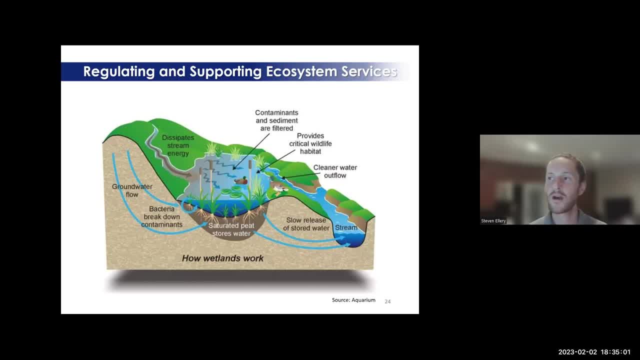 So, very briefly, what are regulating and supporting services? These are services that are provided by wetlands, That assist, for example, in flood attenuation. So you know, one of the big discussions that has happened in the Etiqueni or the Durban municipality recently is how we can revive wetlands. 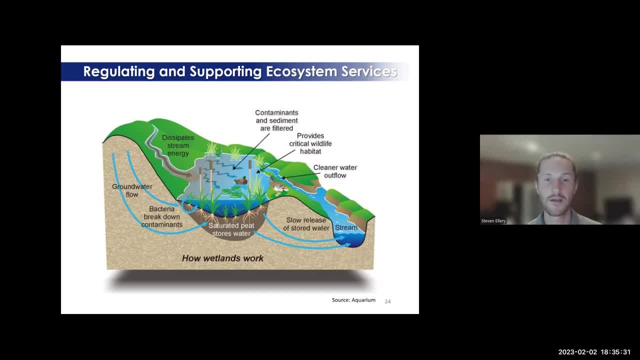 within the municipal land holdings to provide flood attenuation to prevent further floods like the ones we had last year. Malik Aramani- Right 入. And that is a function of wetlands having generally gentle gradients as well as quite robust vegetation that slows the flow of water down drastically. 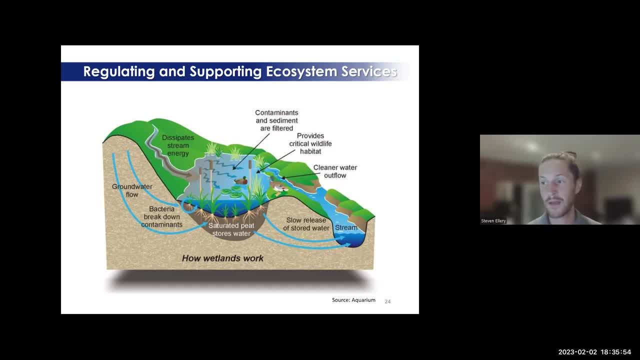 You know, and also, if those stream flows or groundwater inflows into wetlands are polluted for whatever reason, then the nature of the interactions between the plants and the soils in wetlands are, you know, really great at breaking down contaminants. And you know, often wetlands are referred to as sponges, or the kidneys of the world, or great filters. 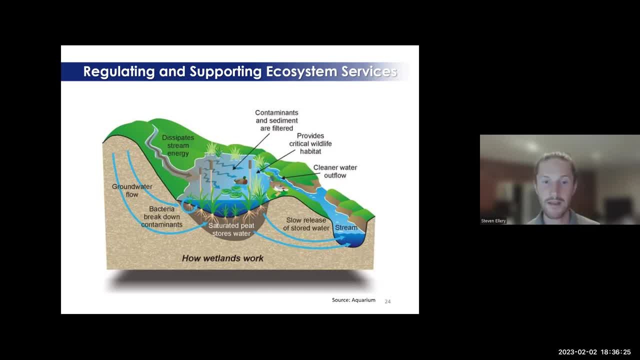 And this is wise, because they are really phenomenal at processing And assimilating contaminants, And they also provide very slow release of water. you know they're often referred to as sponges, so they release water very slowly And so, especially in dry periods, wetlands often remain wet for much longer and can provide stream flow regulation to downstream areas and, you know, provide at least a consistent. 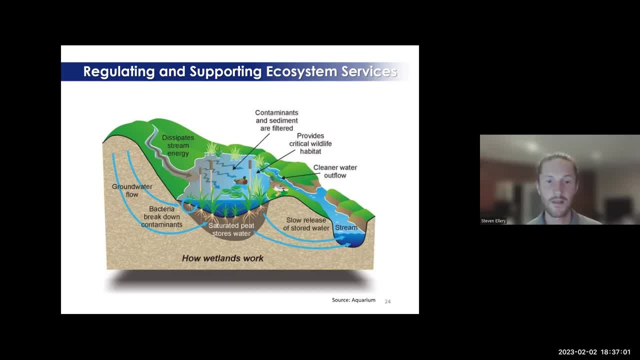 flow of water, And you know provide at least a consistent flow of water. And you know provide at least a consistent flow of water for human use As well. as they provide critical wildlife habitat for many unique and endemic species. 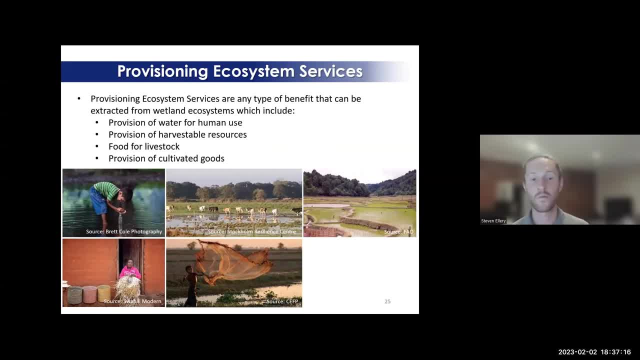 Provisioning ecosystem services. So this is basically what we can harvest from them, what we can derive. So you know water, for example, it's a big one, and lots of people cultivate in wetlands rice paddies, era. you know lots of people cultivate it with lands, rice paddies and. 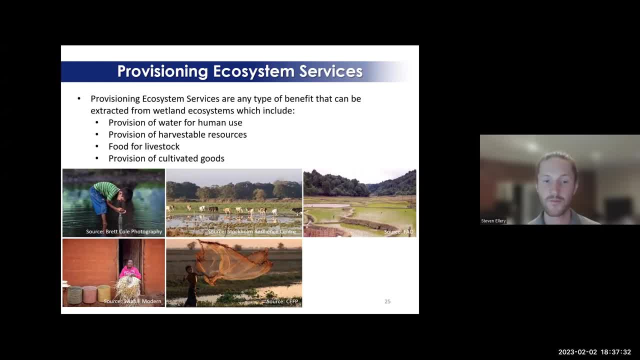 Many madumbis are grown in wetlands as well. You know. there's also lots of fish and just food. They're abundant in terms of the food that is produced And, you know, during dry periods they also can provide phenomenal grazing resources for cows, cattle, 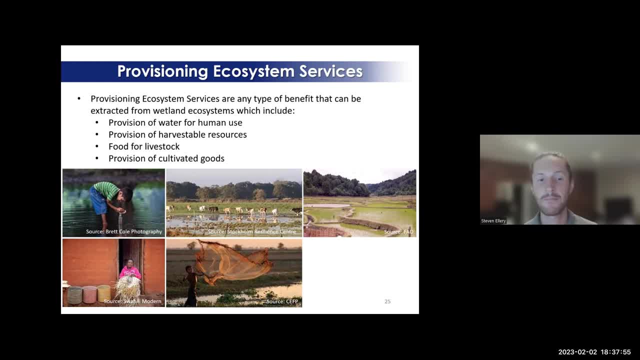 sheep, goats and then many, many reeds. many crafts can be made from wetlands. You know they are abundant in reeds and there's a particular species here in KZN. It's known as ikwane or cypress latifolius. 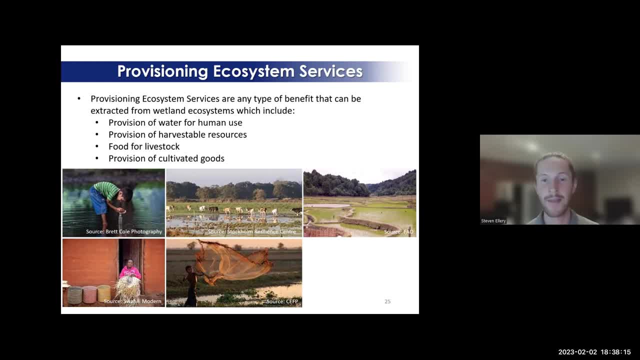 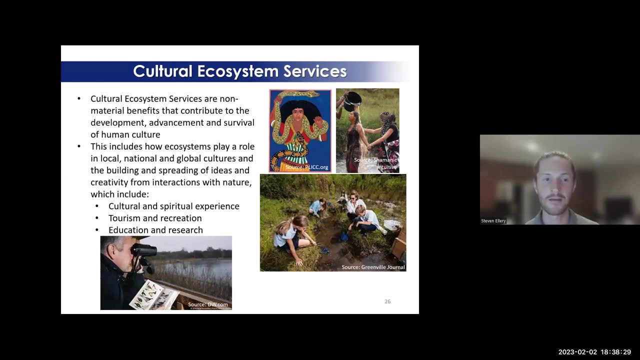 which is used to, you know, make beer baskets and mats and all sorts of things, And so those are some of the provisioning ecosystem services And then the cultural ore Non-material services that are provided, And yeah, and those include cultural and spiritual experiences. 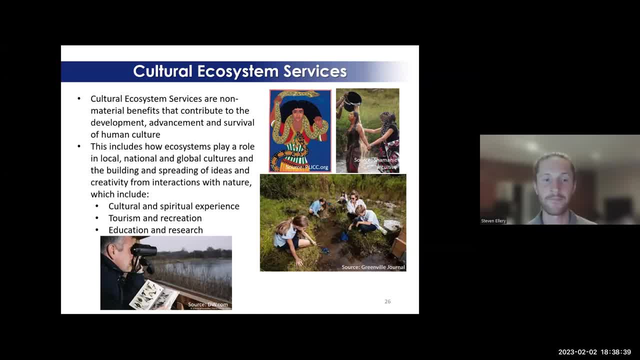 birding, tourism and recreation and, of course, education and research. I recognize quite a few people in the chat. We run lots of wetland courses and we've had a couple of these. I know Tapello and Oki and Pumla have all come on wetland courses. 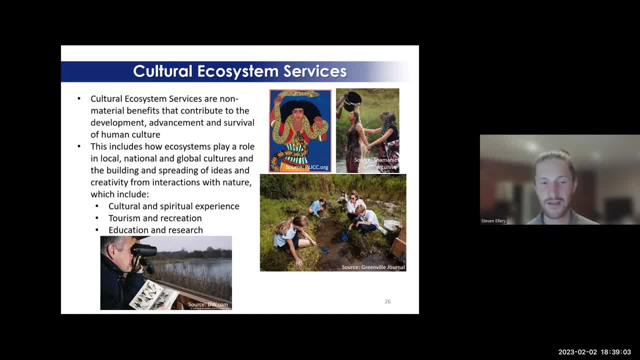 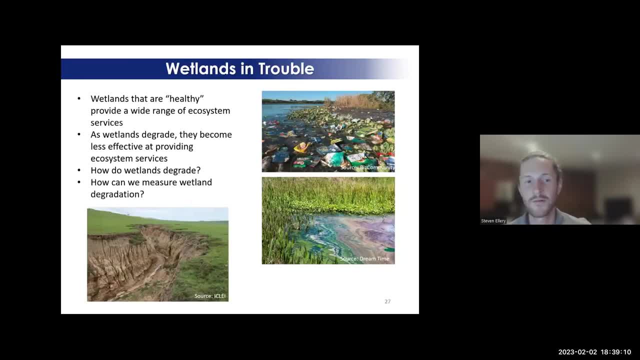 So you know, it's also a great opportunity to be out in nature and learn about what's happening. But of course, with, yeah, our increasing population, our increasing need for land and space and agriculture, we are putting wetlands in trouble. 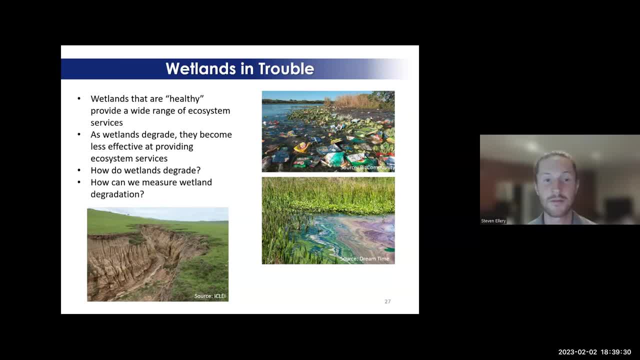 So healthy wetlands can provide a wide range of ecosystem services. But, as I'm sure we kind of know, as wetlands degrade they become less effective at providing ecosystem services. And yeah, one of the key questions that I often address in my line of work is: 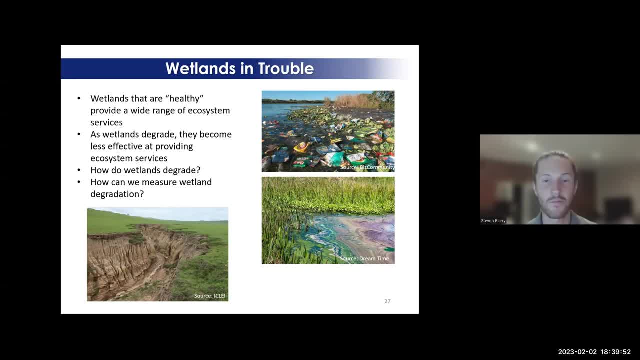 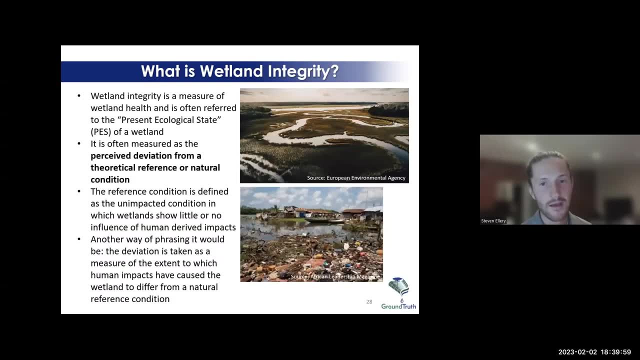 how do wetlands degrade and how can we measure wetland degradation? So let's conceptually think about how. what is wetland integrity? What do we refer to when we think about wetland integrity? So wetland integrity is a measure of wetland health. 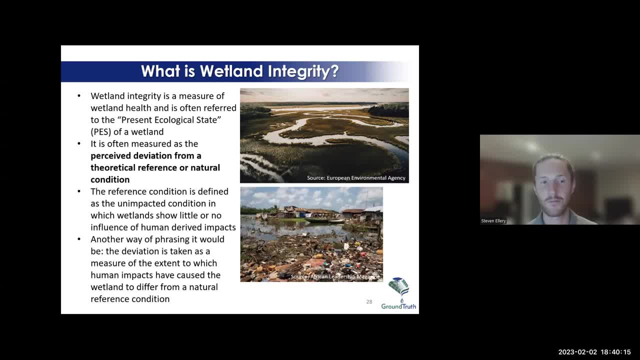 and is often referred to as the present ecological state of the wetland, And this is the perceived deviation from a theoretical reference on natural conditions. So basically, before humans had any impact on the environment, before humans had any impact on the environment. 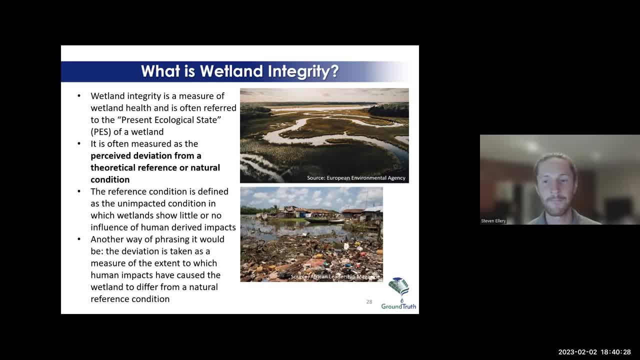 before humans had any impact on the environment, before humans had any impact on a specific wetland, And that can be impacts in the catchment. it can be impacts in the wetland. That is what we call the reference state or the natural condition. 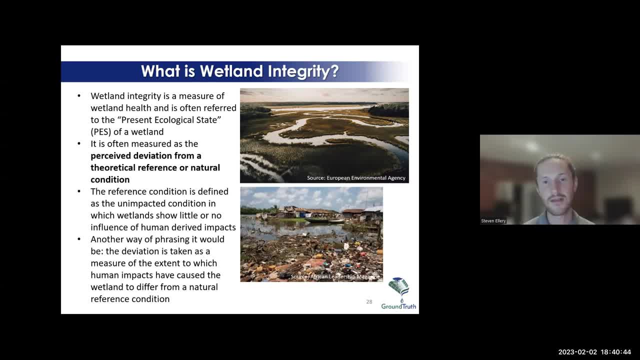 And yeah, so it's a measure of the deviation, or the measure of how much humans have impacted the wetland and how much that wetland now, in its current state, differs from a natural reference condition. So you know how are wetlands degraded? 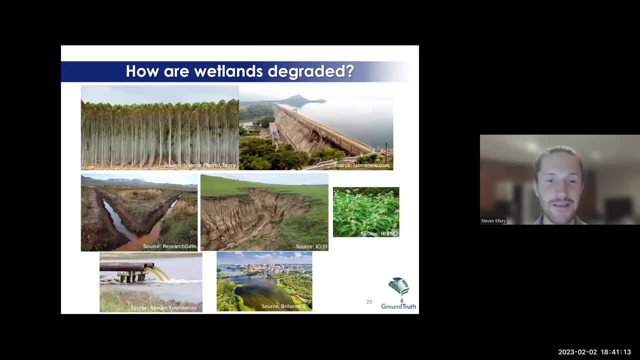 I'm sure you guys can tell me as well as I can tell you, how wetlands are degraded. But if we think about the three components of wetland formation- hydrology, geomorphology and vegetation- we can actually get quite a good sense of how wetlands can be degraded. 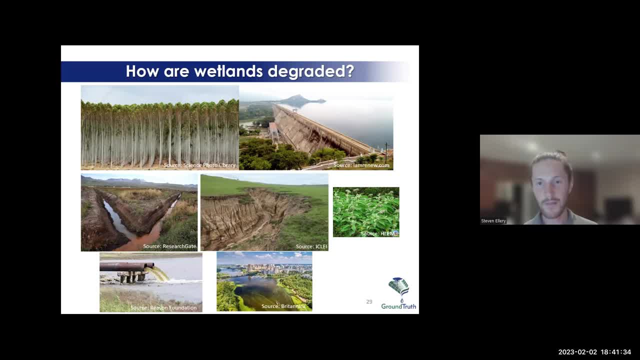 So if we remove hydrological aspects from a wetland through massive gum plantations and eucalyptus plantations, through the constructions of dams, you know immediately we are preventing water from entering into those wetlands. So you know the movement of water through wetlands is. 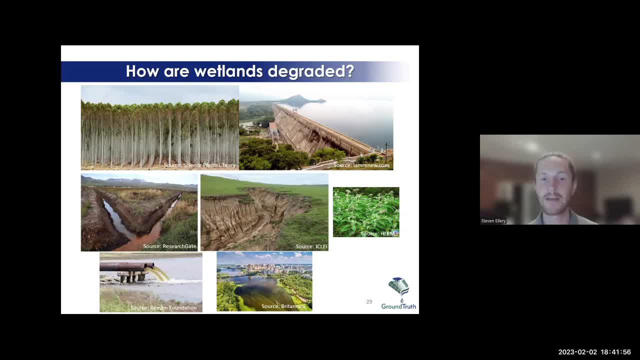 one of their fundamental functions. and if we remove that water, well, we, you know, decrease their integrity in their present ecological state drastically. um. but also, you know, once water enters into the wetland, one of wetlands primary functions is to? um slow water down and to distribute water. 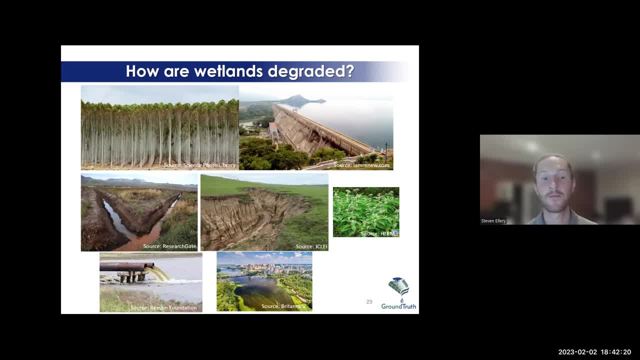 across a wide basin, um, but if there are massive drains that are dug or channels that are done into the wetlands, well, the water is just going to flow into those channels or drains and flow straight through the wetland and out at a much more rapid and pace than what naturally would. 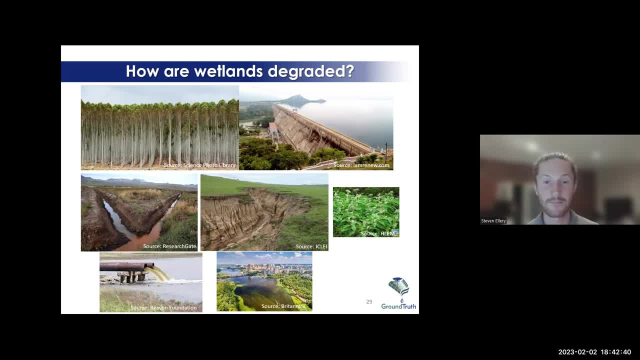 occur. and you know, of course also, um you know i mentioned earlier, and with high levels of grazing, with urbanization, as water flows into wetlands at increased runoff velocities, that can often trigger erosion, um, and you know, the formation of large gullies and dongers and those, those, 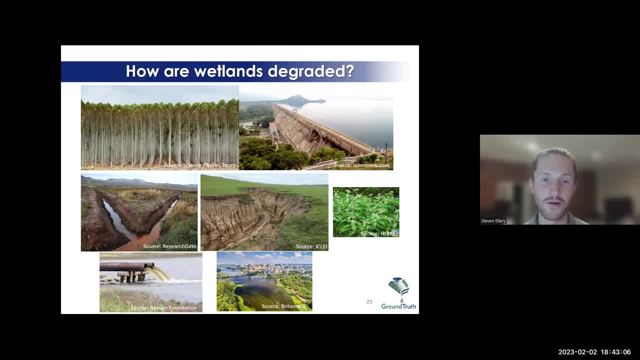 features in a wetland act in a similar way as a channel or a drain and um, and those also result in the um degradation of wetlands. and then, of course, alien plants and the encroachment of- i've got a picture of bugweed there and and bramble or all sorts of alien plants- have a negative effect not only on the vegetation but 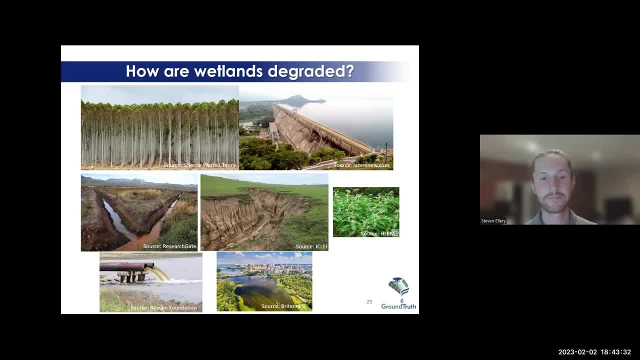 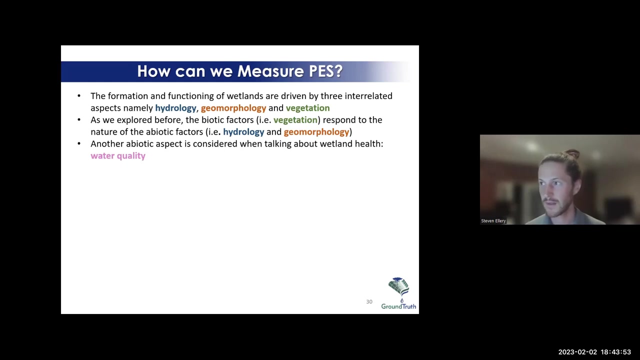 also on the hydrology. some plants, um, as i'm sure we will know, have a much, much more um rapid ability to uh to take up water and then, of course, water quality issues as well. so how can we measure the present ecological state, as we mentioned, the function of which? 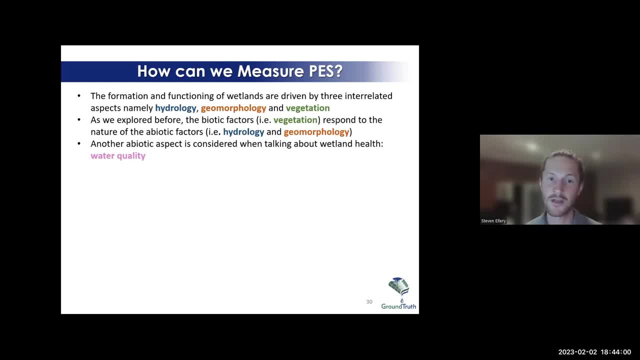 functioning of wetlands are driven by hydrology, geomorphology and vegetation and, as we explored, um you know, the biotic factors respond to the nature of the abiotic factor. so vegetation responds to hydrology and geomorphology and, um you know, another aspect that is considered, another abiotic aspect that is considered. 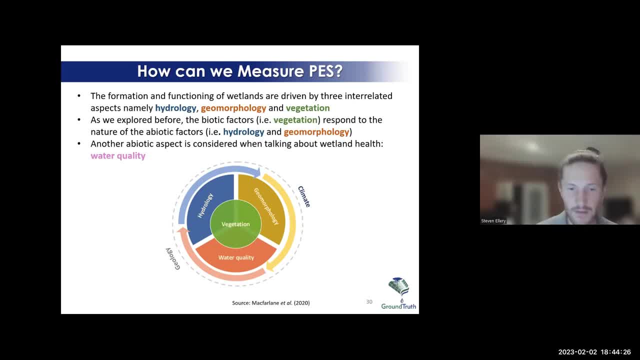 when talking about wetland health is water quality. so if we um take all of this into consideration and we can measure quite accurately now um how hydrology has deviated from its natural state, how geomorphology has deviated from its natural state, how water quality um 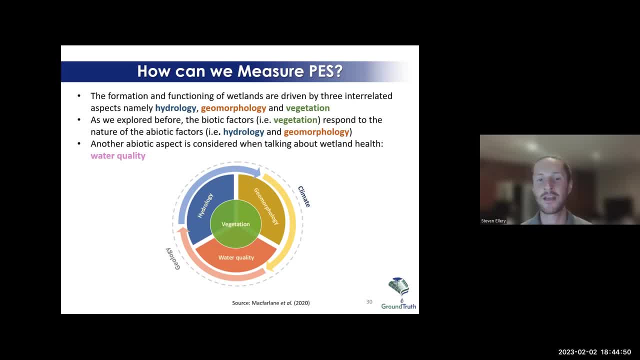 has deviated from its natural state and how that is all affecting vegetation and how the vegetation composition of a wetland has deviated from its natural state, and we combine all of those factors together and to come out eventually with a present ecological state. so, um, in conclusion, i know it was quite rushed and it's still quite fast. 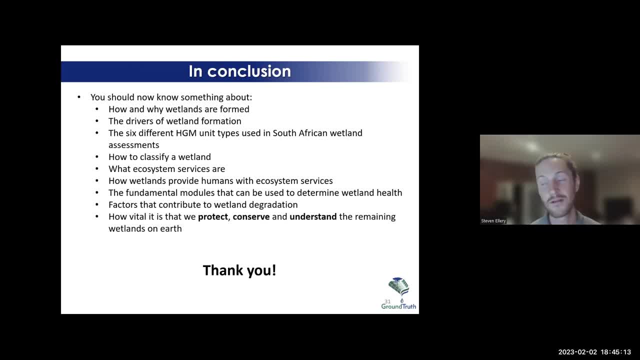 but you should now know something about how and why written are formed and drivers of wetland formation, as well as antibiotics. know something about how and why wetlands are formed and drivers of wetland formation as well as. and drivers of wetland formation as well as. Anderson's name is growing in this area, so we should be talking about the contribution ofѤ1 tamarind wateranced to veryososotonan watergasavati解 lanes. all of that we're and I have to do. we let this off the ground off with all this kind of kinda subject. 문ic on the end round. 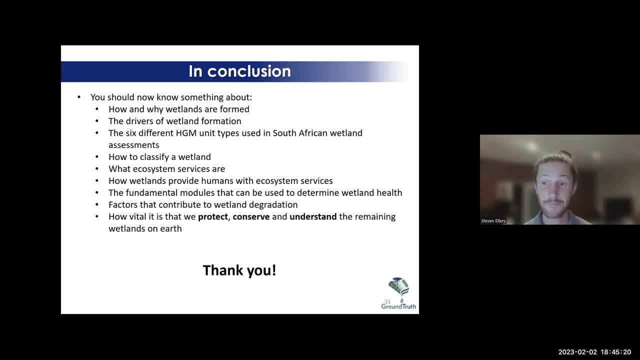 as something about the issue in your types, how to classify a wetland and what ecosystem services are, um, as well as what, uh, ecosystem services wetlands provide to humans, and as well as factors that contribute to wetland degradation, and, yeah, and i guess just how vital it is that. 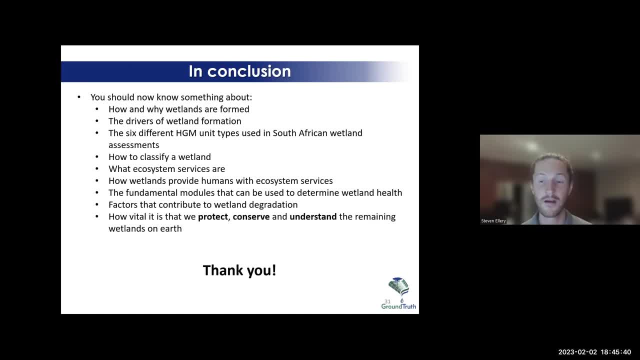 we protect and conserve and understand these systems, because they are completely priceless, to be honest, in our landscape and we really, really need to um be more active in our um just consideration of them in our landscape, and and so i thank you all for your interest in in science and 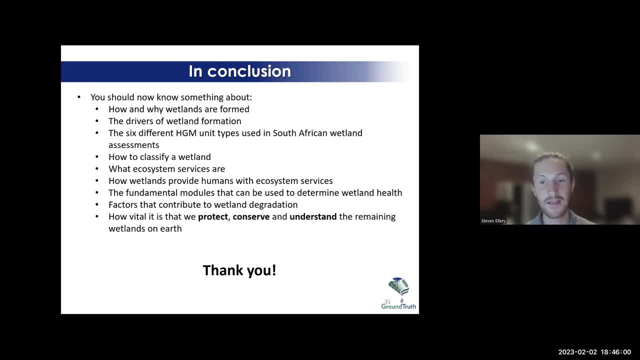 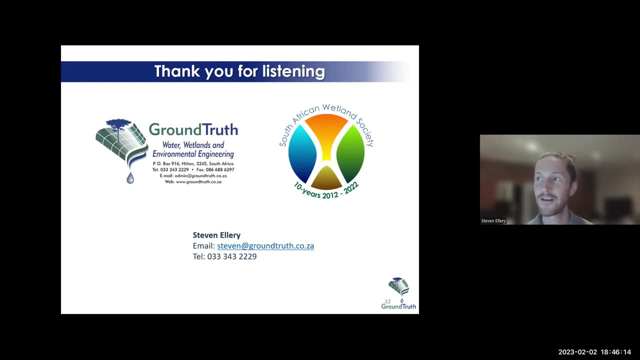 wetlands and understanding these systems. it really is um heartening and it really is encouraging to know that that there are people out there who are interested and and really care. so thank you very much for listening and if there are any questions, please feel free and um, yeah, thanks, thanks for being here, great. 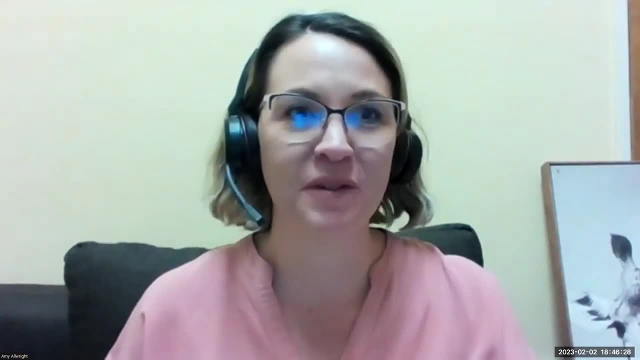 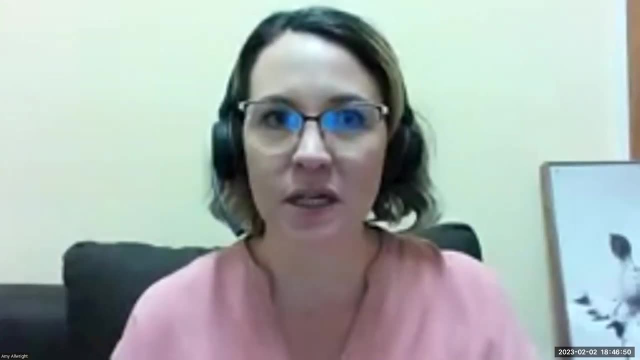 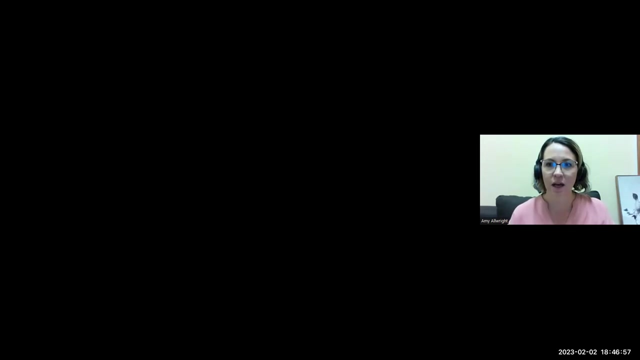 thank you very much, stephen. um, everything was very clear and, uh, i really enjoyed the presentation. cool, um, but please, if you have any questions or would like to um chat to stephen, please feel free to put your mic on or type a question inside the chat. um, i see there is one question already. um. 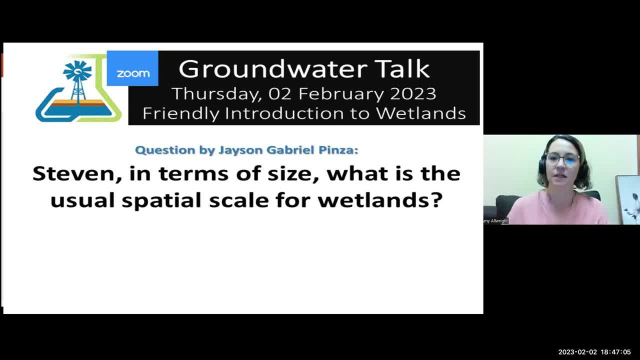 it's a question from jason um asked to stephen in terms of size, what is the usual spatial scale for wetlands? good question, jason um, but to be honest, the, the these systems are so diverse in their nature and you can have, uh, a system that is is really small and in the case of, maybe, a depression wetland, there's no such thing as a. 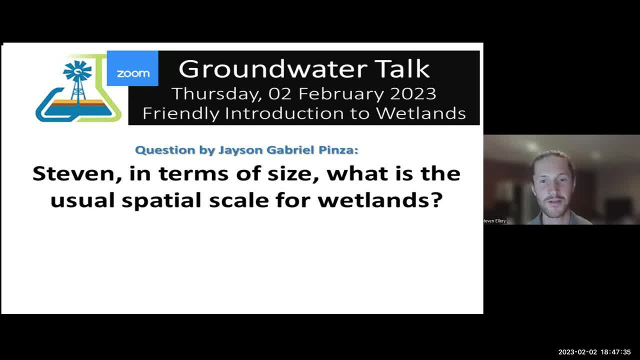 wetland. I did my whole master's thesis on a depression wetland that was maybe 300 square meters in total, But then, you know, the Amgeni Flay is probably 250 hectares big at least. So it really depends on the HGM unit type. So typically the seep wetlands. 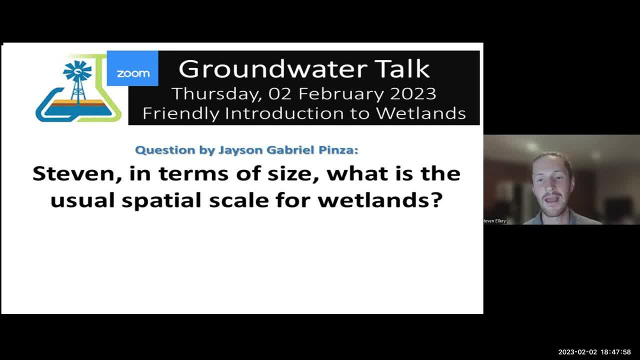 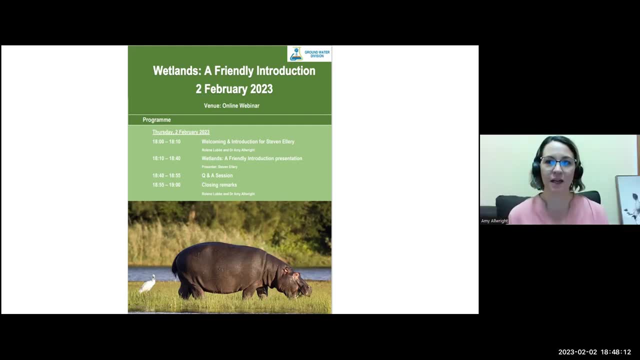 the wetland, flats and the depression wetlands are smaller And then typically the valley bottom wetlands actually occur over a much broader scale. Great Thanks, Stephen. I think that answered that question very clearly. There is another question here from Libasing. 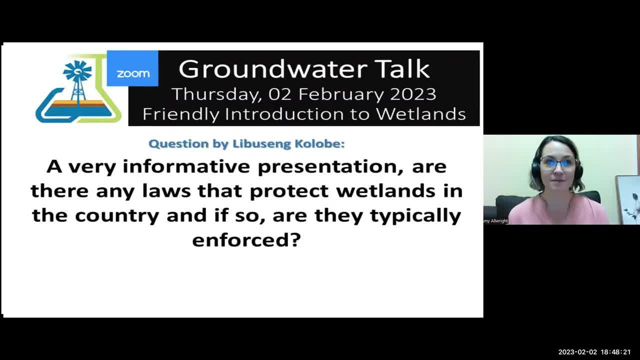 She first comments and says a very informative presentation and then asks if you know if there are any laws that protect wetlands in the country and, if so, are they typically enforced? Also good question. Thank you, And yeah, there are actually. South Africa has great. 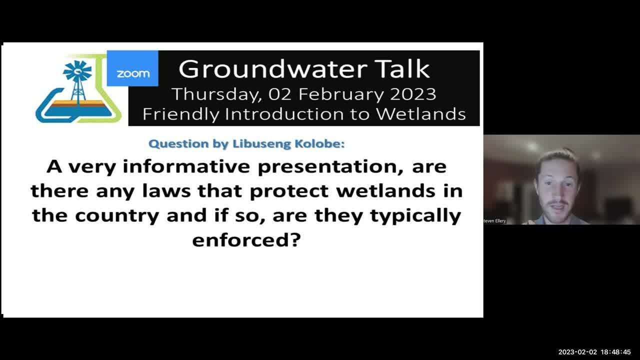 legislation regarding the protection of wetlands And in the last maybe five or six years I think people are slowly catching on just the importance of wetlands in South Africa And so, yeah, More and more of those laws are being enforced and more and more, And you know, just in the last 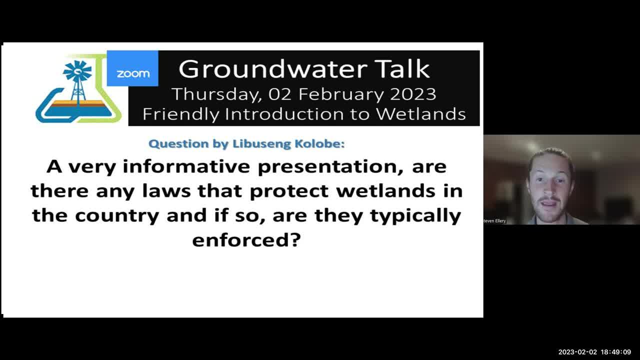 three years, me myself and my company have been called on to a lot of what we call compliance projects, where someone has done something wrong in a wetland and someone has reported them And that person is actually made to rehabilitate that wetland in some way, And so 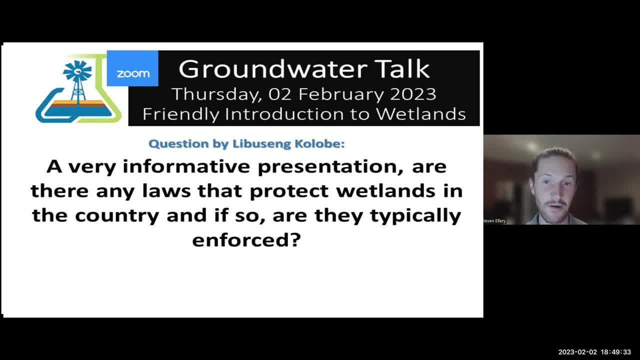 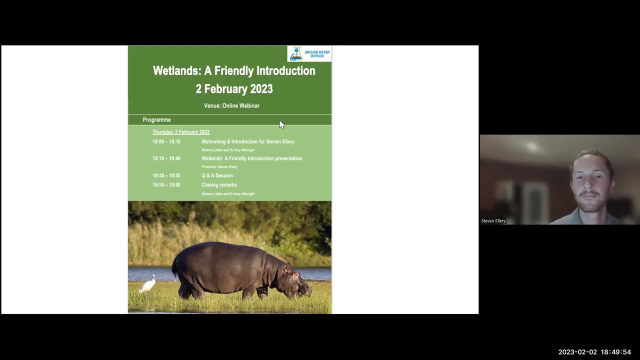 there are actually more and more, encouragingly so, the enforcement of those laws, And those laws are in the Environmental Management, National Environmental Management Act, so NEMA, as well as the National Water Act, and they are quite detailed and quite good. I hope that answers the question. 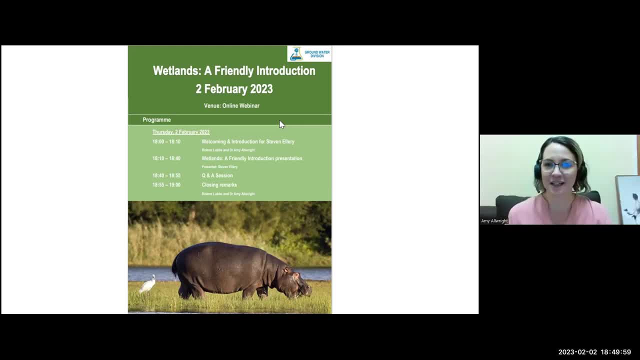 Very interesting. Yeah, Sorry, I was just jotting something down, It was something, that was something. I was just very interesting to hear that you're having compliance work now, people being forced to to remediate wetlands. that's awesome. yeah, um, there's a few more questions, so, um, finest. 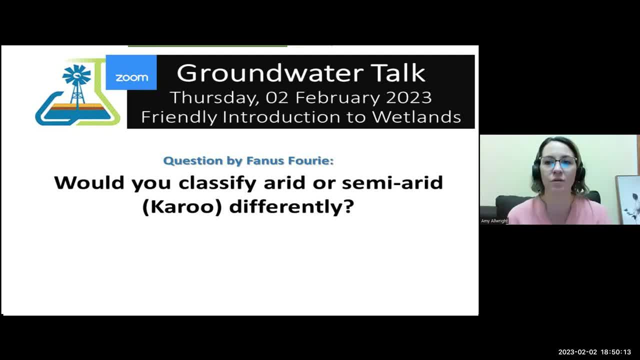 classify arid or semi-arid, something like in the kuru, differently. um. so there's a whole, uh kind of sub, sub field of practice in wetland science, which is wetlands in, in semi-arid and arid areas, and i did my master's thesis on a wetland in a semi-arid. 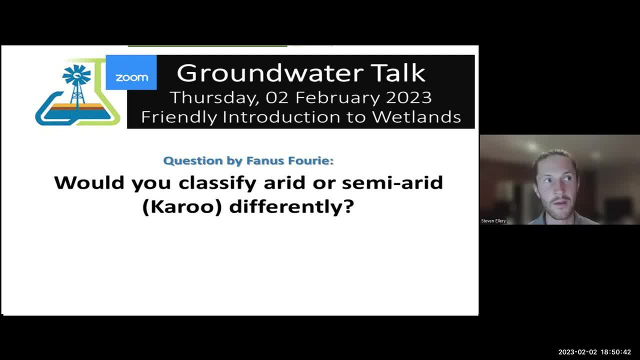 environment and that wetland was only, you know, um, yeah, it was only wet for two or three months every year, um, but because it has been wet for two or three months every year for um about, i think we estimated the age of the wetland to be about 1.3 million years old. 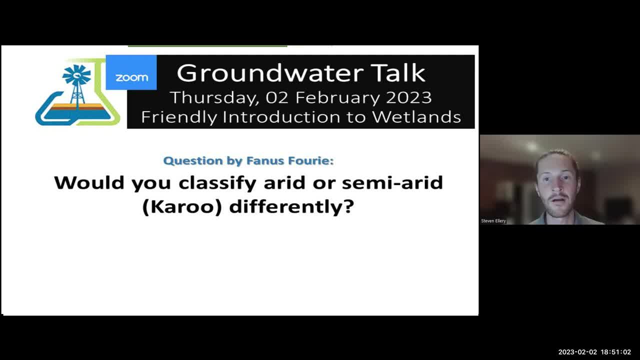 um, you know, because it has happened for that long, the soils are indicative of a, of a wetland, and but you definitely get different soil indicators and different vegetation indicators in arid and semi-arid environments and and you you don't necessarily classify them any differently, but you certainly treat them differently when you are assessing them. 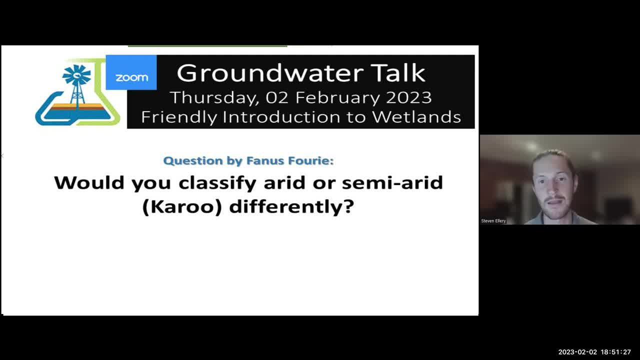 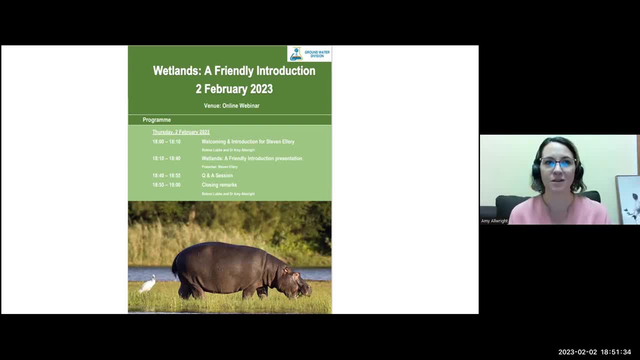 and you certainly treat them differently when you are rehabilitating them or restoring them, and you, you don't necessarily treat them differently when you are rehabilitating them or restoring them. well, that's interesting to know. i, i i guess off the top of my head. i would wonder in those sort. 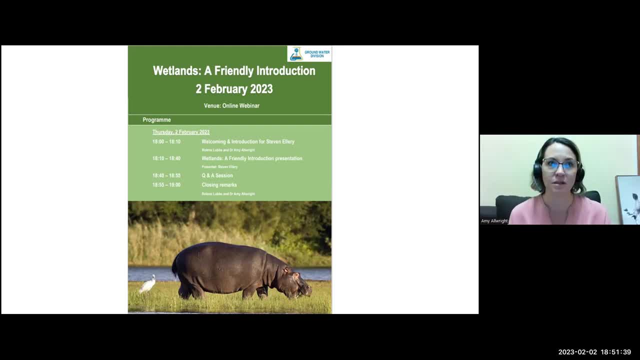 of environments if groundwater plays a more substantial role because it's not as much, you know, surface runoff in terms of precipitation. but that's just often. often in those environments actually, um, wetlands act as groundwater recharge points. okay, because the water table is so far down. yes and um, they are. 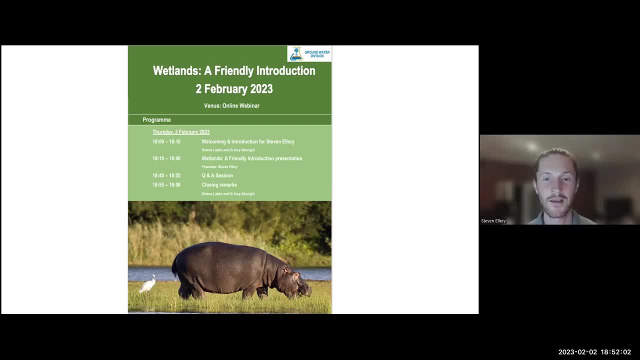 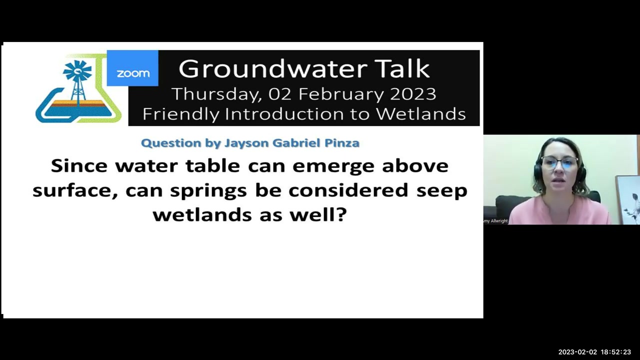 often precipitated, primarily precipitation driven, and and and they, they really don't have any. um, yeah, there's little groundwater upwelling, it's mostly recharge, interesting. um, i see we've got a few more questions here. jason uh also asked: since the water table can emerge above surface, can springs be considered sleep wetlands as well? absolutely, and. 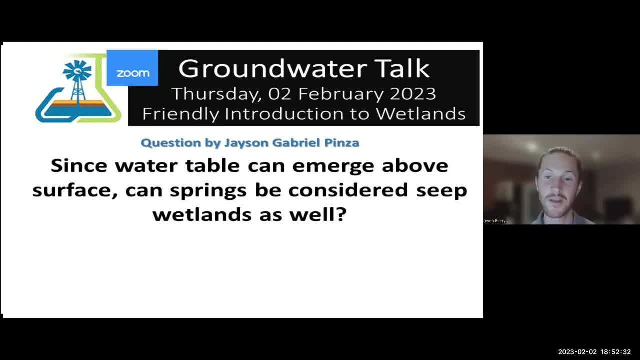 yeah, i think there's a lot of uses, but but i think you know what you could say is for um, for um. you know, as a wetland, as i said, temples are a spring um, but you know, if you go to a common um, often um see wetlands, you will find springs at the head of them or at the uppermost. 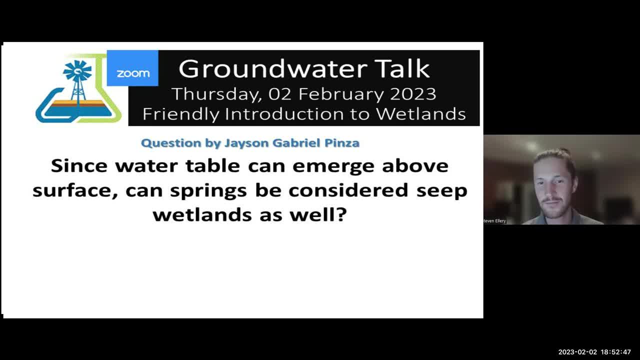 point, and that's, you know, the point at which a separate land often starts, is a spring and, and, yeah, so you know, as i said, there's all these groundwater, surface water interactions that are fairly poorly understood. um, and it would be really great for for, um, yeah, more, more work to be done in. 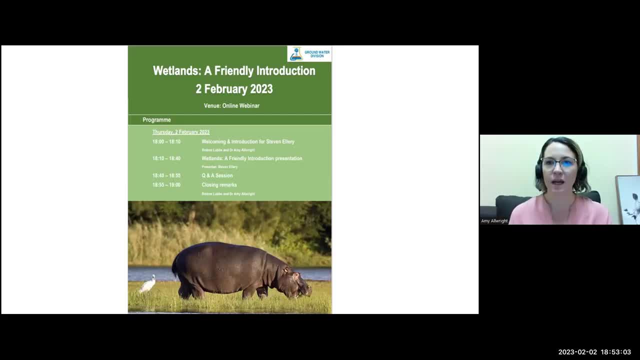 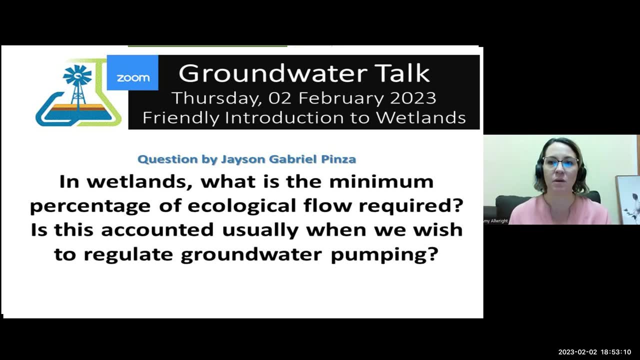 Jason also asked in that question. he says: in wetlands, what is the minimum percentage of ecological flow that's required, and is this accounted usually when we wish to regulate groundwater pumping? yeah, that's also something I want wanted to ask because I know you can't really have a borehole within a certain distance of the river and I assume that there's a similar. 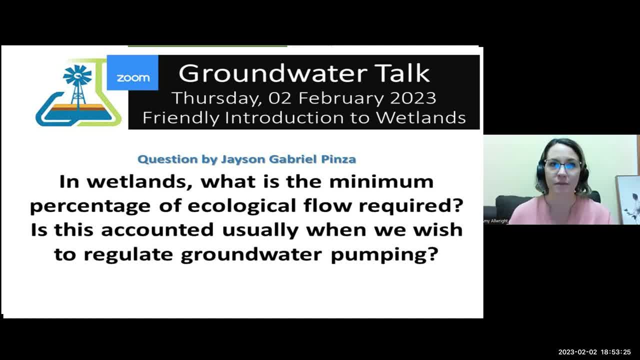 regulation with wetlands? yeah, it's a great question, Jason, and you know, in terms of a minimum percentage of ecological flow, again, you know, I wish that I had a better answer for how that groundwater surface water interaction occurs. we've just been involved in a large ecological 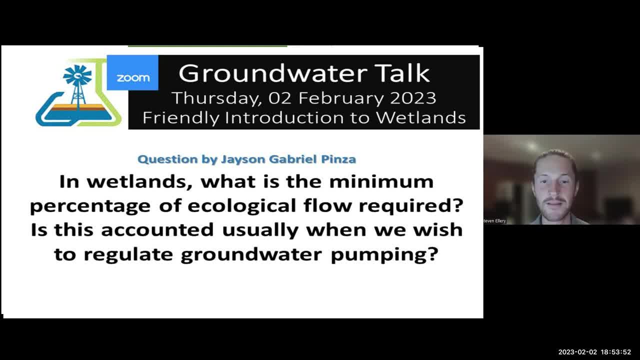 flow study and for the upper orange basement, and we've been asking ourselves the same question: well, how do you factor in, you know, the regulation of groundwater pumping in specific areas where we don't actually know what the groundwater surface water interaction is like? so, as part of the study, we've had a 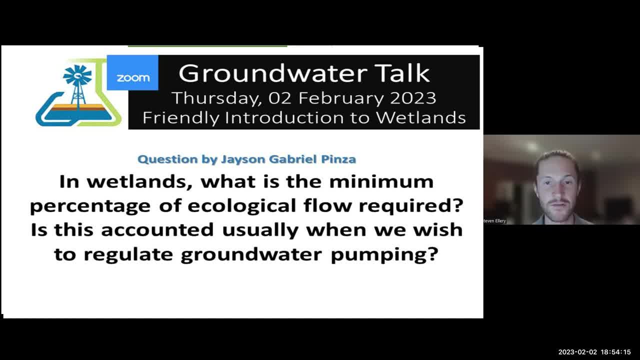 groundwater or geohydrological survey done and it was found that the aquifer is quite far the wetland. so in that case there wouldn't be as much a regulation on the groundwater pumping for the sake of the wetland, because it's not necessarily, it's not reliant on the groundwater. 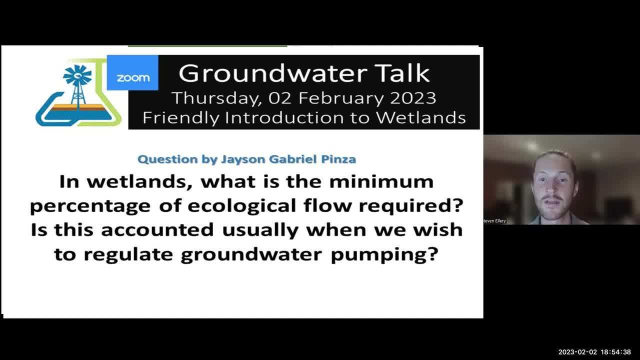 but if that groundwater area falls into a strategic groundwater source area, then there would be regulations against um pumping and from a groundwater perspective, and again, i think it needs to be taken on a case-by-case basis, on a wetland by wetland basis. so, and you know just, 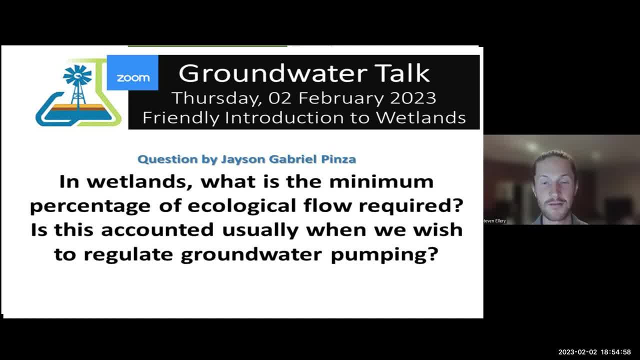 to understand the groundwater, surface water interactions and then to be able to, um, yeah, and determine what ecological flows should be stipulated and in those, in those cases. yeah, so not really an answer, right, but um, more just, uh, um, alluding to the fact that we need more research. 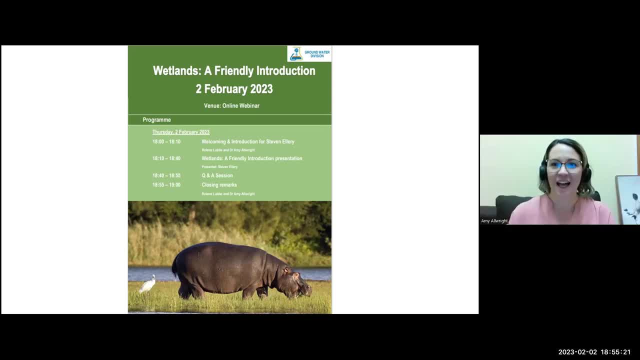 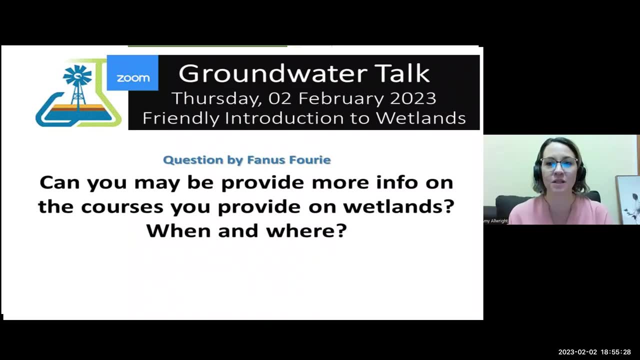 yeah, not one size fits all, right. um, uh, farmers asked um. can you please provide us with some more information on the courses, um, on wetlands that you give when, where? absolutely, um, so we provide. at the moment we have three different courses and one's an introduction to wetlands, so quite, 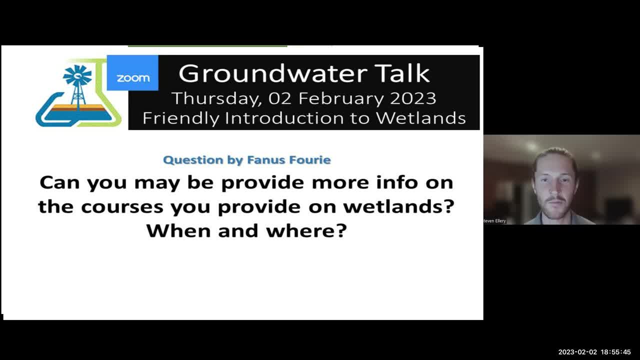 similar to what we've covered this evening, but in quite a lot of detail, and then we do a an assessment course as well, so where we um kind of teach you how to really assess a wetland for its present ecological state as well as its um provision of ecosystem services, and and then 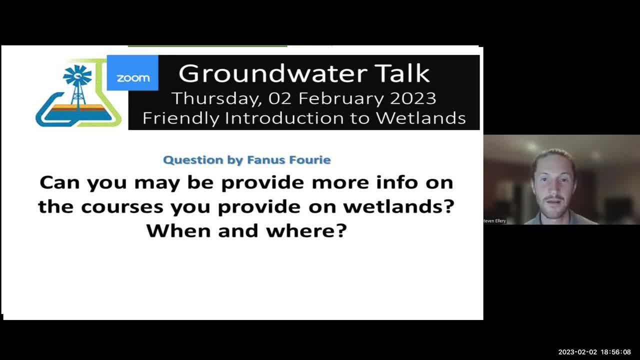 we also go into some of the legislation regarding wetland and mitigation and management, um, and then we also do a wetland vegetation course and and that's kind of more niche for those who are wetland ecologists. and if you send me an email and just stephen groundtruthcoza- 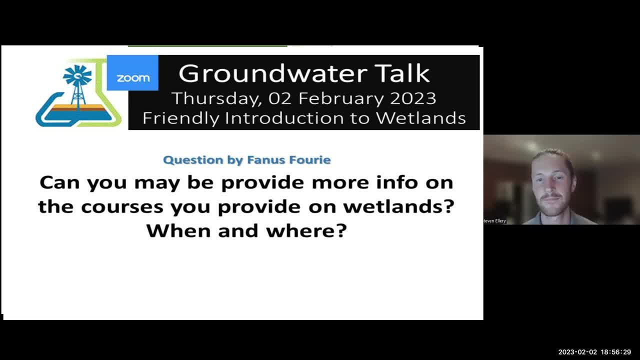 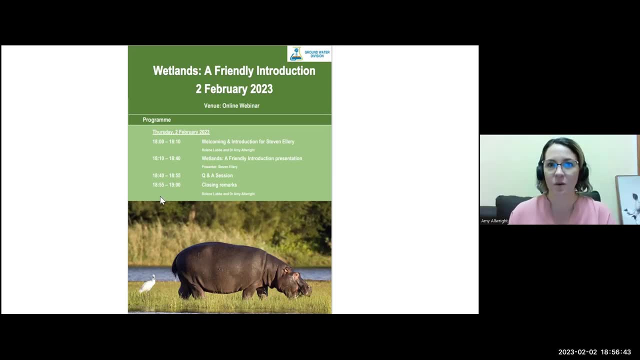 i can provide you with all of that information, and we run them online as well as in person. so there's the hybrid, so you can- yeah, cool, stephen. can i ask you to just jot down your email in the chat, just for anyone that, yeah, wants to get it? 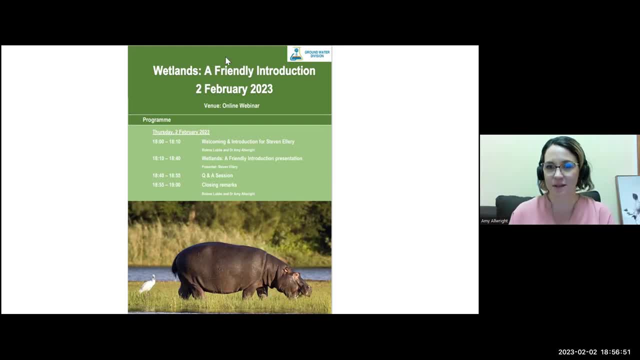 really, do you want me to read your question or do you want to ask it? um, i think i'll rather ask it. then it's going to go quicker. um, okay, so we know that wetlands are very valuable in terms of fauna, which is protected by nema, which is the environmental. 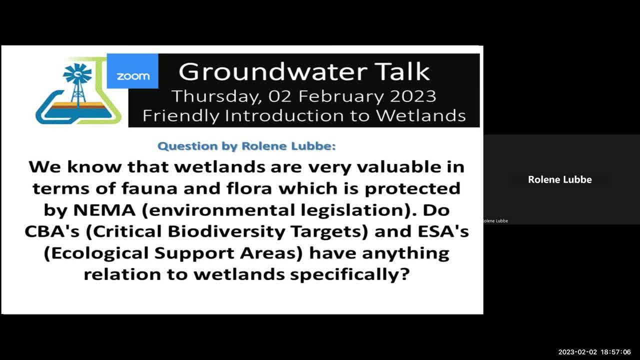 legislation, um. hence why we are celebrating world wetlands day and do cvas, your critical biodiversity areas and ecological support areas, have anything in relation to wetlands specifically? so, um, absolutely um. we have a? um, a wetland specific vegetation type, um and um, and i'm sure you you've uh heard of the? um freshwater ecosystem priority areas. there's. 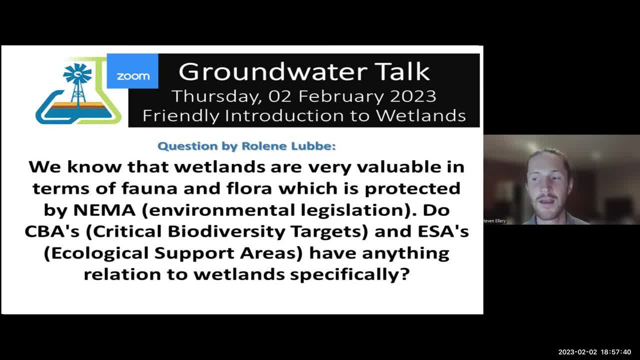 a wetland version. there's a river version, a wetland version of that um, and i'm sure if pumla is still here she'll be able to talk about the um work that sambi is doing on the national wetland map six um, and so there's actually a, a massive map of all the wetlands in south africa. 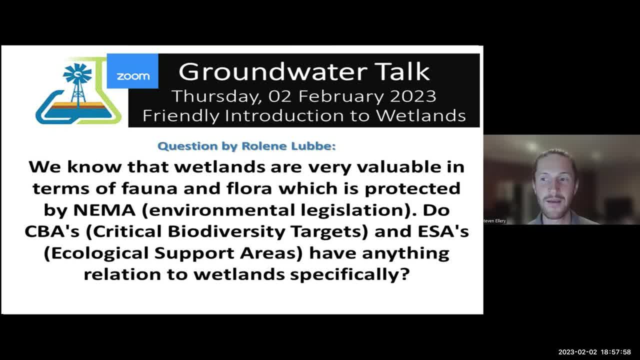 and well, a lot of them anyway- and that that layer takes into account, um the critical biodiversity types of the cbas. it takes into account the um support- ecological support areas- and um. it then basically comes up with a threat status of each wetland type in the. 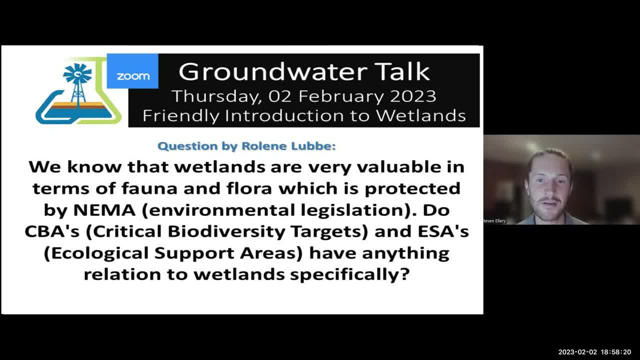 way that um you may describe, such as the gdps and the first wetlands, um, and so therefore, the uh, the, the um, the information that we have is a bit different than what we normally should talk about and while it's um, it's uh, it's in its um, yeah, it's in its vegetation type, which 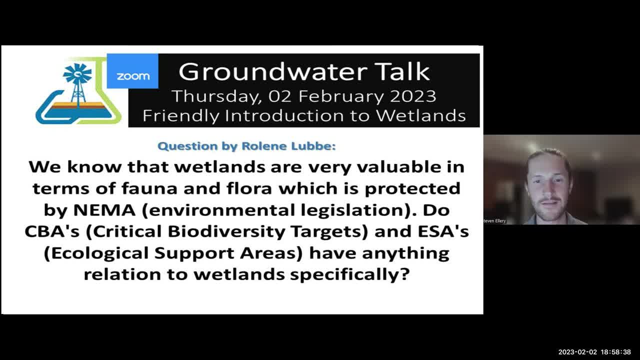 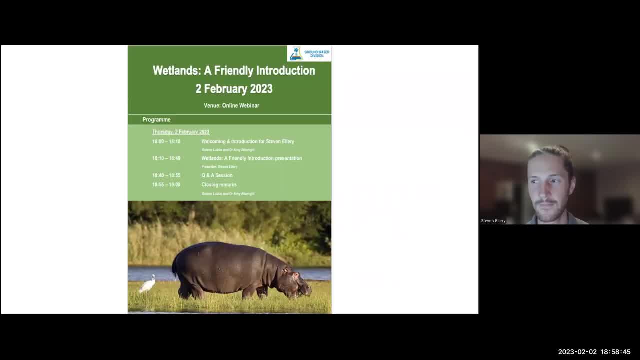 is tied quite strongly to the cbas and the eas. um, so there is um, yeah, and, and we have to include information about that in all um wetland reports that we write. so we have to, we have to do our home, this, um. one last comment here from putti. uh, he's asking me: can you elaborate on how to distinguish? 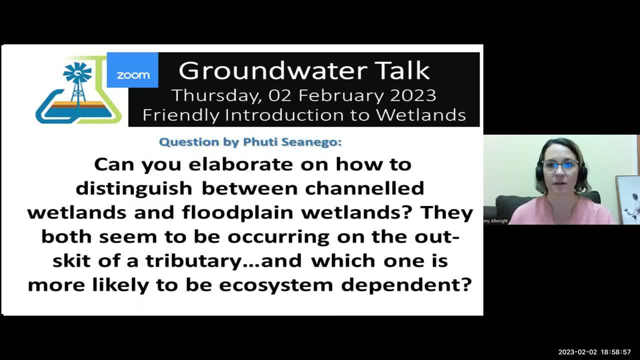 between channeled wetlands and floodplain wetlands. they both seem to be occurring on the outskirts of a tributary, and which one is more likely to be? um ecosystem dependent? okay, um, if well, i understand the first part of the question fairly well, um. 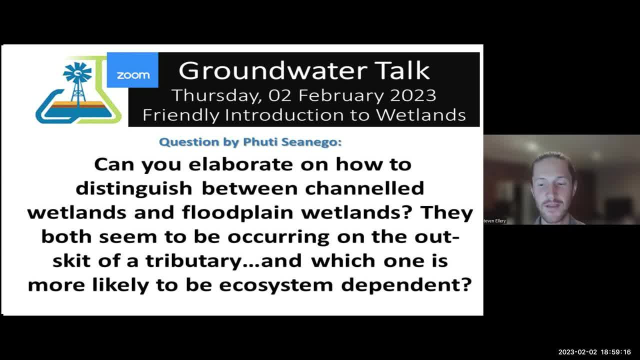 um, this is a good question and it's something that, um, it can be quite challenging to identify and and it's a pity that i didn't include the floodplain um hgm unit type in my presentation because, you know, the floodplains have very distinguishing features and generally they 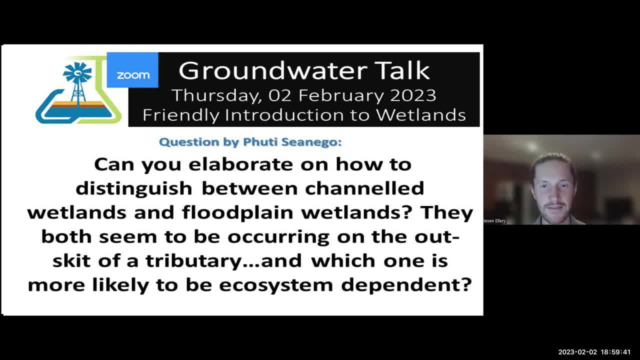 have much bigger catchment areas, and that's a general rule. it's not not um, always the case, but because they have generally a much bigger hydrological load coming in, they- um, you know the channel course inside a floodplain will often evulse and change. so then what you start seeing? when the course of the channel changes in a floodplain, you start. 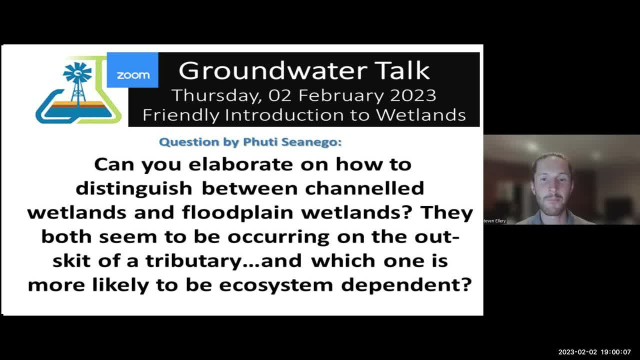 finding these um abandoned channels and backwater depressions and oxbow lakes, um, and those features are really only found in floodplains um a channel valley bottom generally has a quite a shallow channel in its natural form um and it doesn't have those distinguishing features like oxbow lakes. 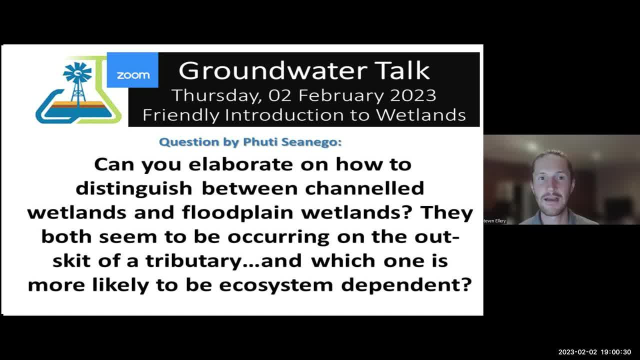 and backwater depressions and yeah. so it's hard to explain that without illustrating it and without showing it, um, but that that's one of the um biggest distribution factor, factors, um, and then maybe, if i um understand the second part of your question, um, so they, they do both. 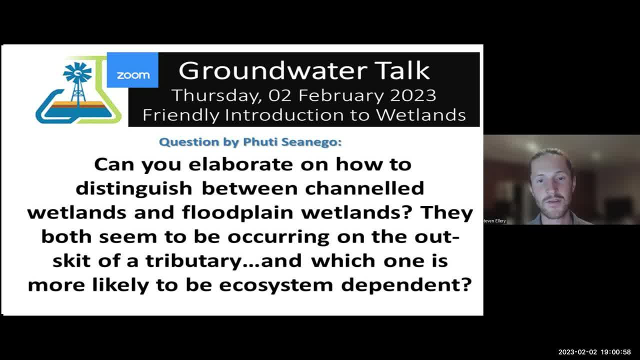 occur along a river channel, and so you know they are characterized by a channel, and that flows through a wide basin, and and so you know there are many geomorphic factors that lead to the formation of a wetland in those contexts. um, and so that's one of the things that i wanted to talk about, um. 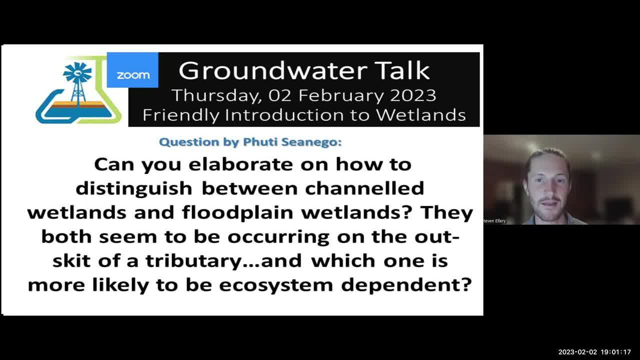 and but one of the the predominant factors is that it's a channel, um that enters into a flat and broad valley bottom, um and with that, when there's flood waters, that water is able to get out of the channel and into the kind of adjacent wetland, um and um. yeah, i hope that answers answers. 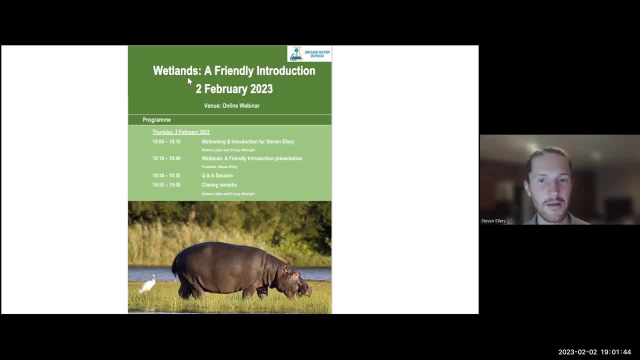 your question. if if i did not answer, maybe you can clarify what you what you want to ask. uh uh responded and she says: uh pretty also says: thanks, steven, he's happy. uh pumla also says: you explained the nwm and just to add that it is constantly being updated. 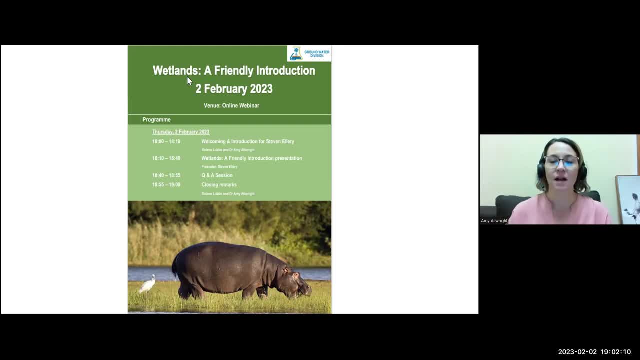 and improved. as there are so many areas in south africa where wetlands have not yet been mapped, sure he's going to step up in the way that they already are. i am looking forward to seeing you there. um, um, um, um, um, um, um. all the thanks, steven. um, i'm grateful that reline found you and that you were willing to to give the. 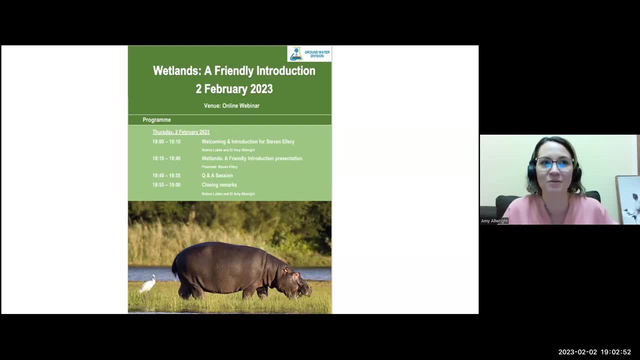 talk, i definitely learned something. i know you know wetlands, you know it can is influenced by groundwater, but it's not something we like specifically think about very often. um, so i thank you for that. and then uh, and we have your email, so if there are any more questions or uh, 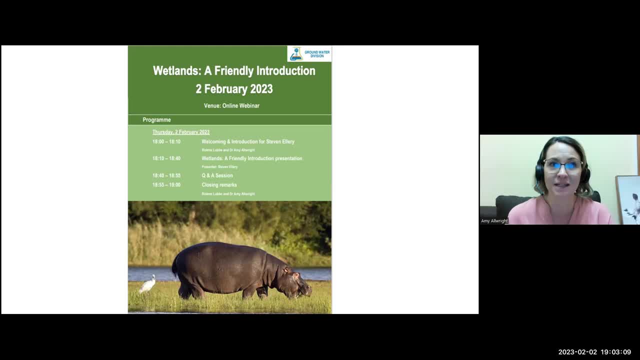 people want to um speak to you about consulting or attending some of the courses. i'm sure i can send you an email and um and then reline. is there anything that you want to do do? thanks, steven. um, i just want to thank steven on behalf of the groundwater division and the unprofessional 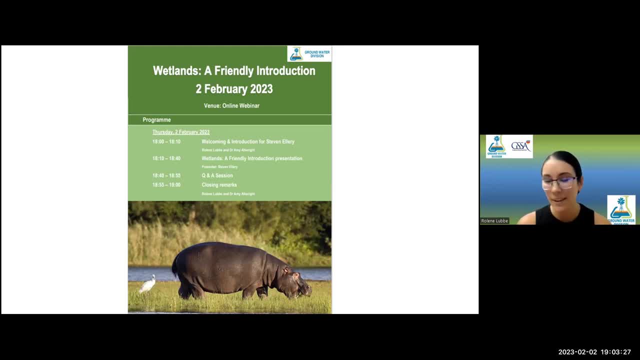 society as well, and thank you for your time and thank you for clearing your schedule and the wonderful presentation that you presented. i feel that most or everyone now understands what wetlands are or just have an introduction on it and how important they actually are to groundwater and seeing the gap that there is for groundwater.